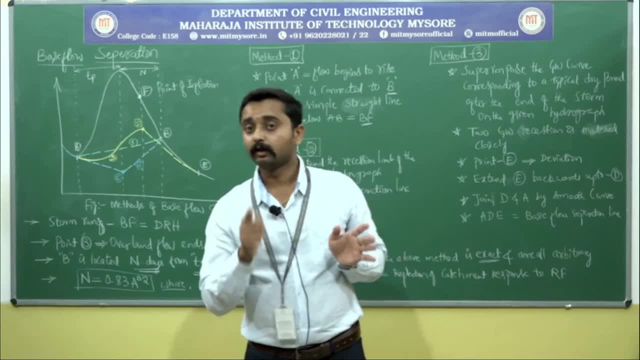 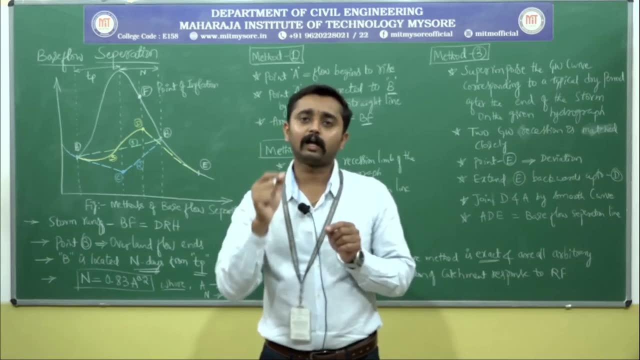 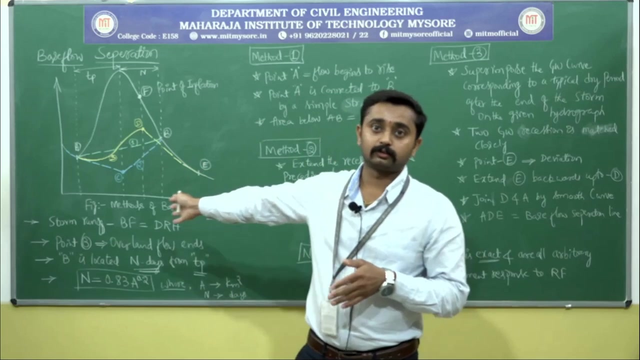 we must separate the base flow. Why? Why we need to separate the base flow? Because base flow contribution is very low. That too, it takes years together. It takes more time period to reach the nearby stream and the quantity from the base flow is very low compared to. 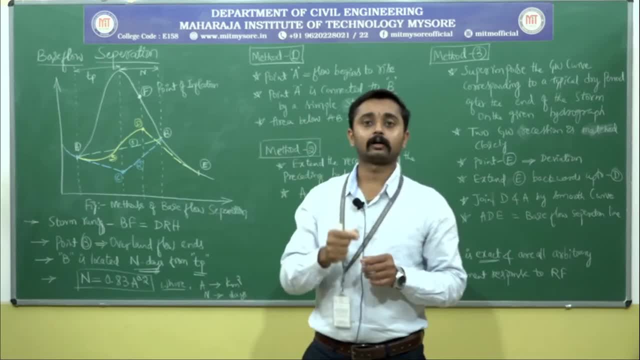 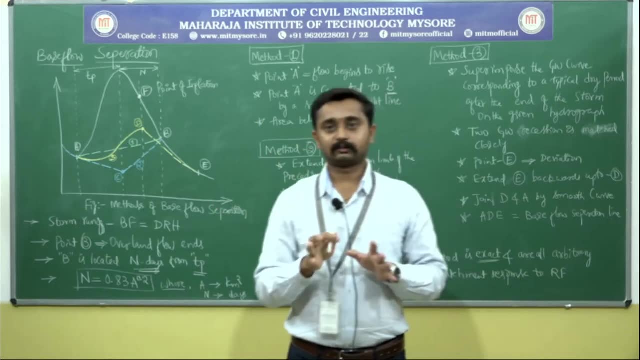 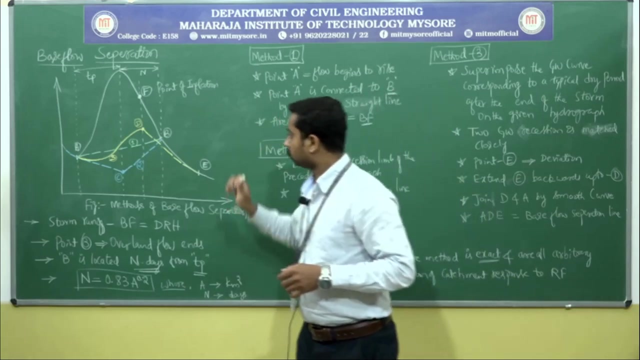 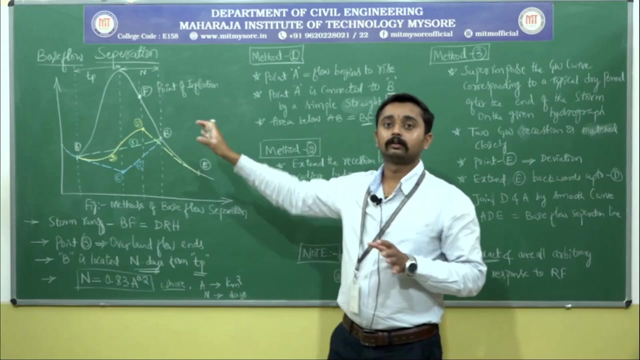 the surface runoff. That is why, while preparing hydrograph, we must separate the base flow. There are actually three methods to separate the base flow. I will explain one by one each. First of all, this is the single peak hydrograph for an isolated storm. 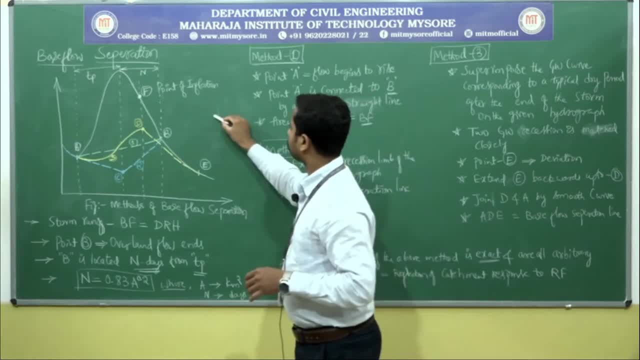 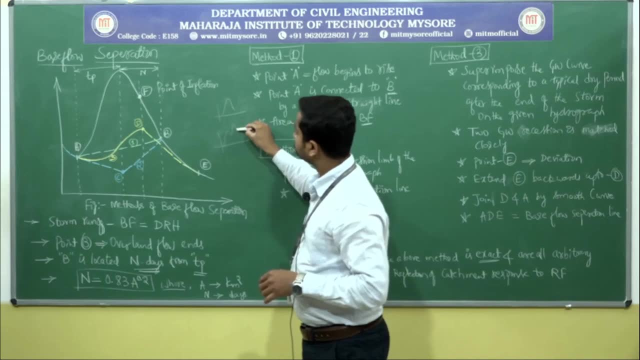 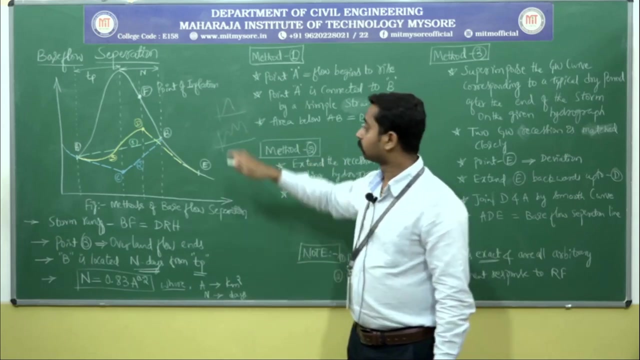 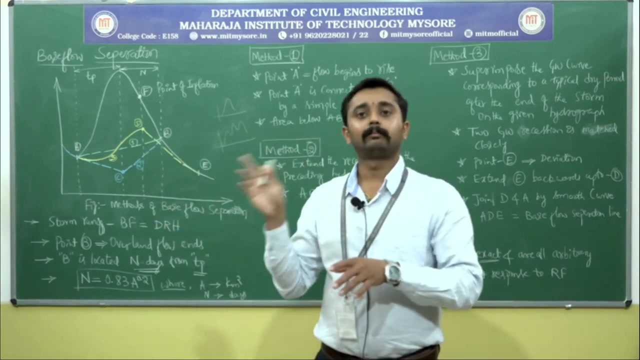 Very simple: Isolated storm, Single peak. If there is a complex storm, then there will be multi peaks. For isolated storm, there will be single peak hydrograph. For complex storm, there will be multi peak hydrograph. So this is. I have taken single peaked hydrograph Now. 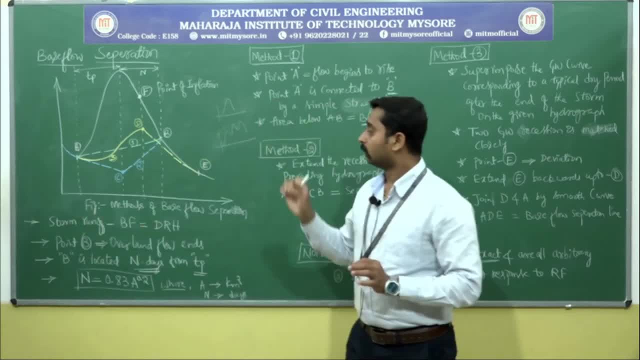 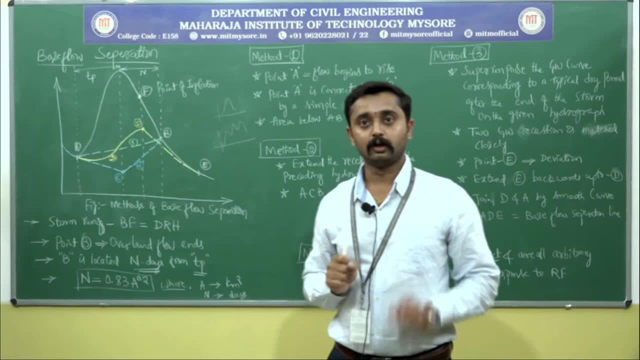 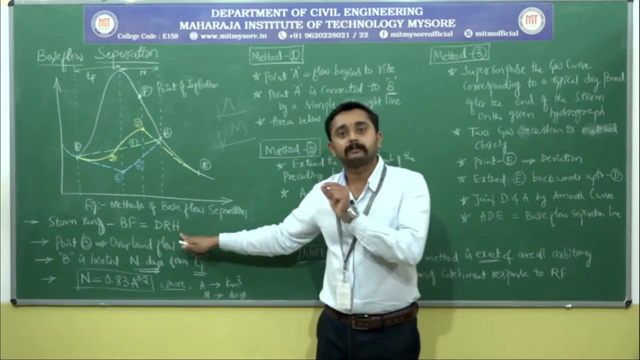 listen. the first point: what it says, Storm runoff minus base flow, equals to direct runoff hydrograph. Yes, of course. in the last class we studied: In order to obtain the direct runoff hydrograph, we must subtract the base flow. We must subtract the base flow from: 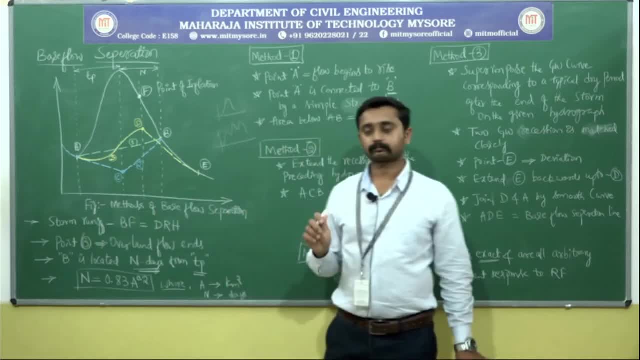 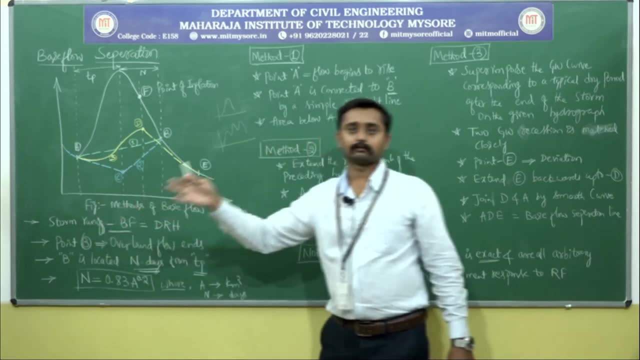 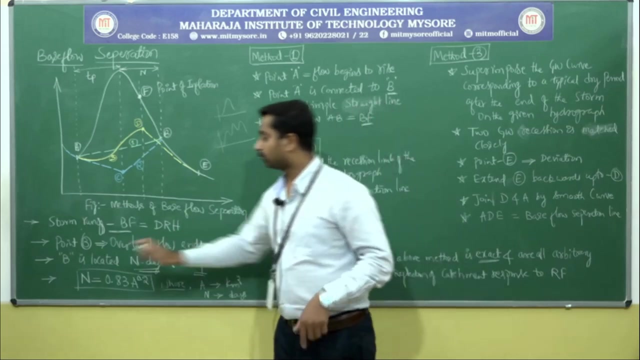 the total runoff. That is what storm runoff We must subtract the base flow from the storm runoff. What is storm runoff? Nothing but runoff, surface runoff, direct runoff, in order to get the direct runoff hydrograph. What is the second point, Point B? This is point. 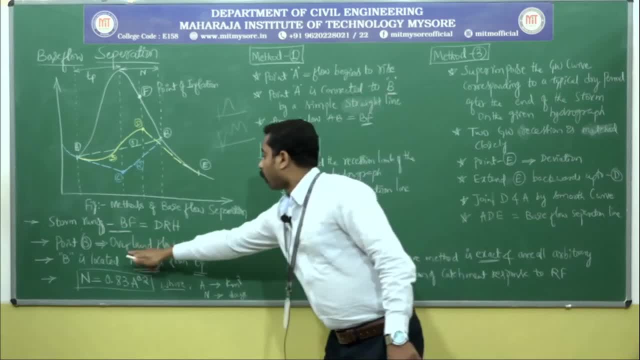 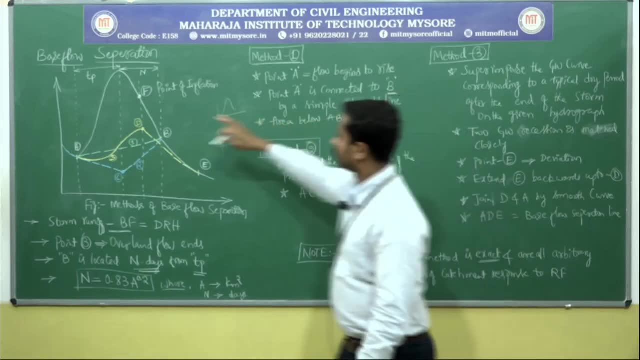 B represents the over land flow ends, The end of the over land flow. This is the hydrograph. So this point B represents the end of the over land flow. Over land flow means The over land flow. This is the hydrograph. This is the hydrograph. 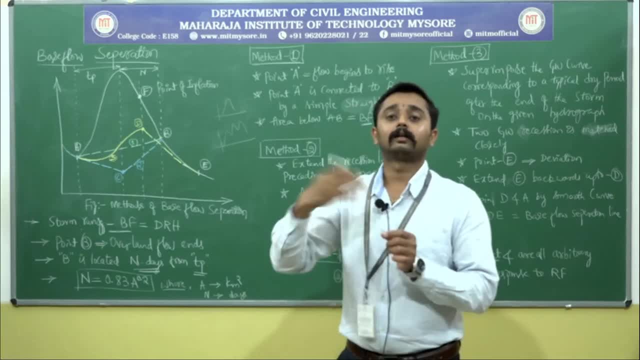 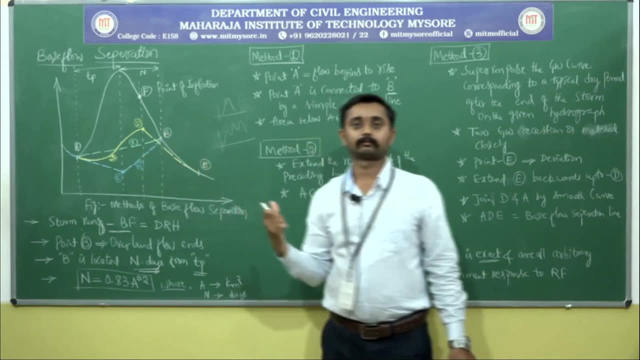 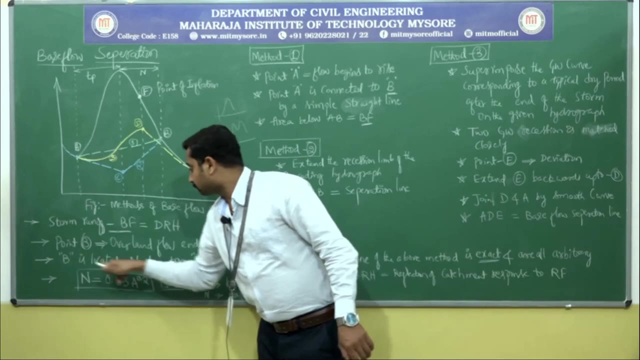 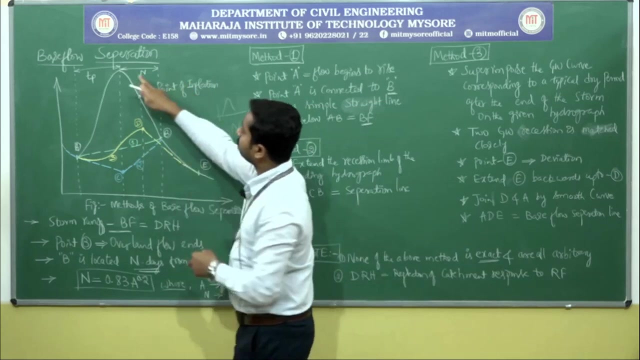 end of a point in a denote murder there. hang it there. the runoff is contributed from this point. from this point, the contribution of base flow acts. okay, this is all about second part. next one is being located. my go, the point B is located and days from TP, and that this is the point B is located from, and days. 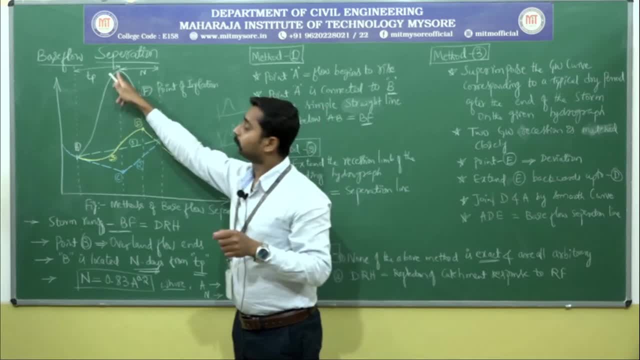 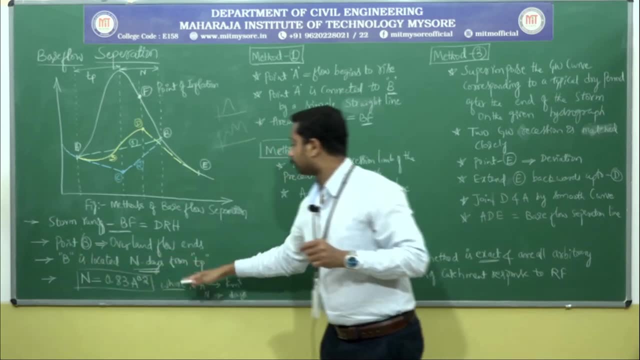 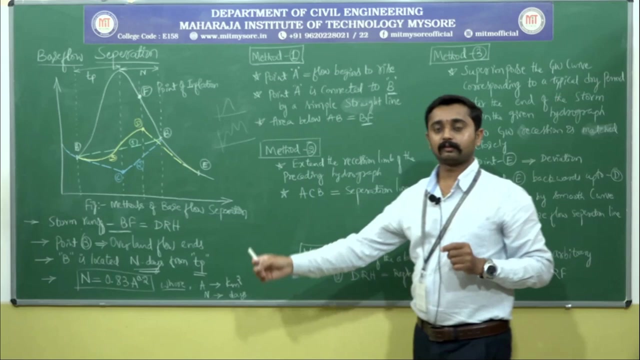 from s, from where? from peak of the hydrograph. okay, this is point B- is located and days from TP, nothing but from the peak of the hydrograph. and there is one empirical formula for that. N is equals to 0.83 a power: 0.2 n is: 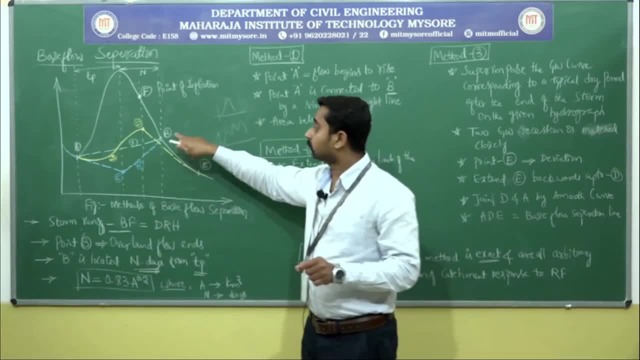 equals to N is for locating the B, n is equals to 0.83 to defined as 1. point 6e, the topic. okay, this is the fourthting factor in here that is going to encanting focus. so, at last, point a of the caso' of the manger through thatowana ours nurse is going to. most likely that happen. give you some haste. if you are from from MD now look at this: how often need any single piggy? and yeah, this much��고 workload on instrumentich align. align this one. so. 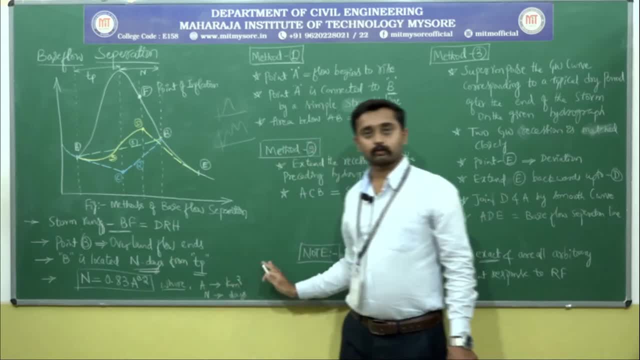 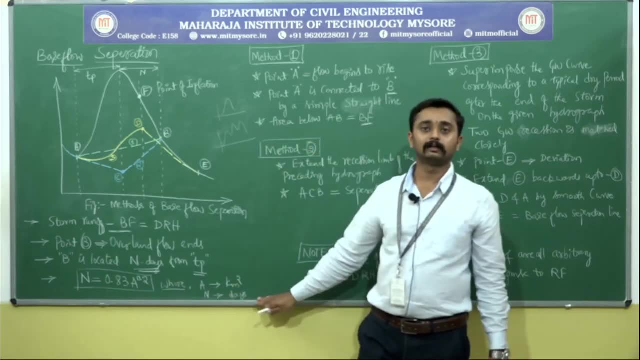 that, for sweet humour, we, as good rosé cano, cutting in rushing or in several into a power 0.2 where a is in kilometer square. if we put the area in kilometer square, then we get n value in terms of days, then we get n value in terms of days. this is empirical, for already. 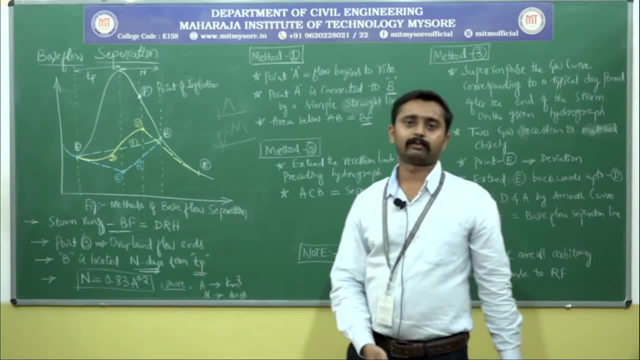 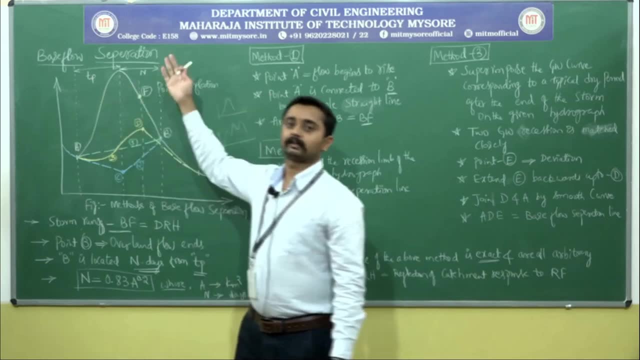 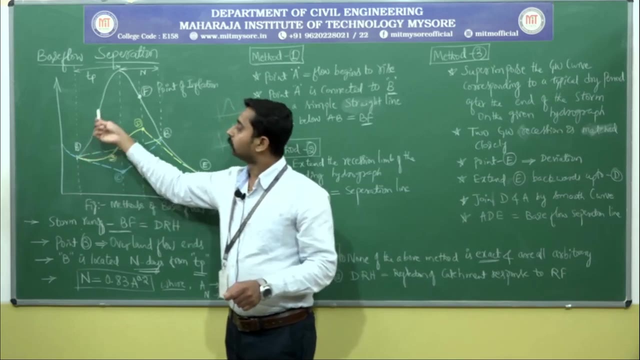 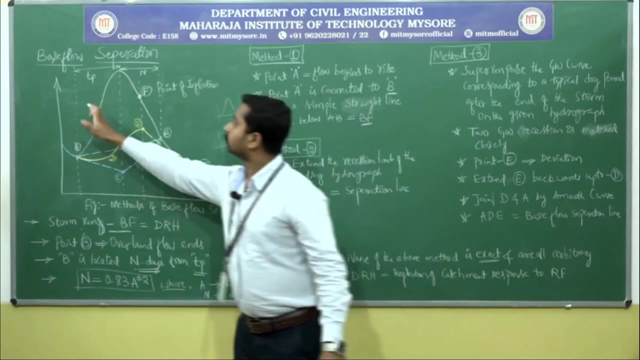 derived already, standard, one empirical formula. okay, and this is about the basic things. tp, nothing but time to peak from the point a, and this is the point where runoff is slowly rising. so from this point, from this point to the peak, is tp. that is time to peak from the initial point in the peak. 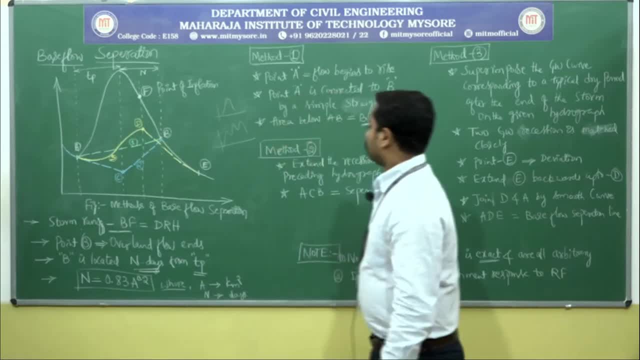 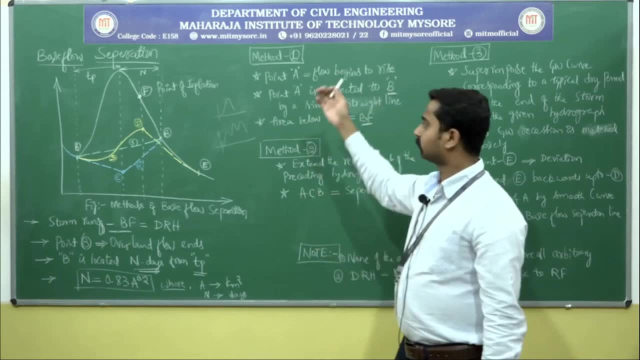 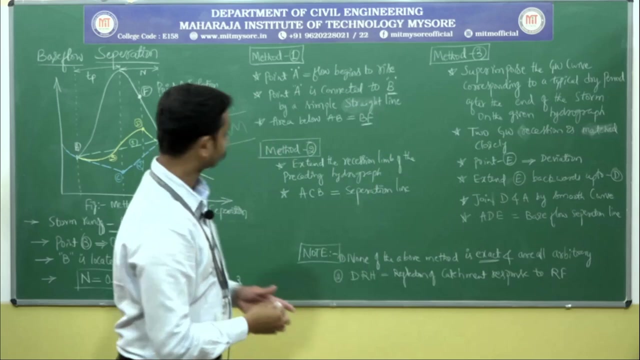 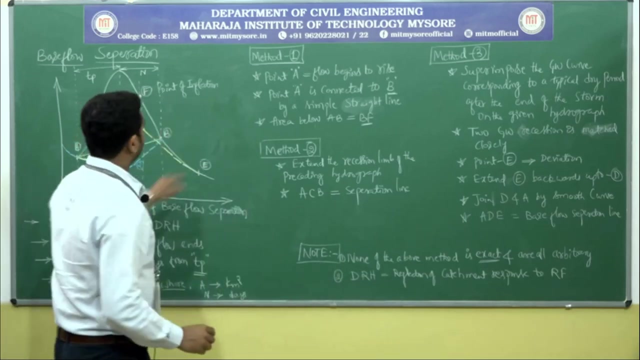 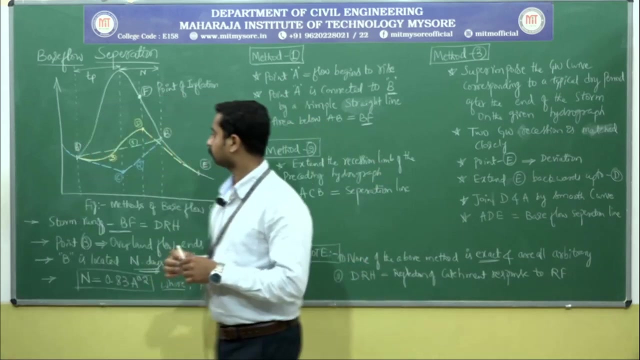 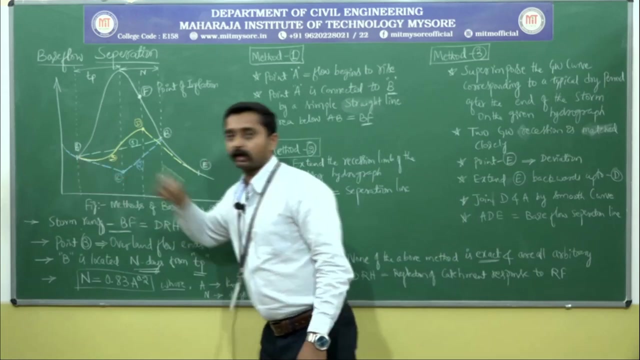 the time required is tp. usually there are three methods in order to separate the base flow. that is method one, method two, method three. method one is a very simplest form among all these three. okay, method one. listen carefully, method one, what it is, point a equals to. this is point a is equals to: 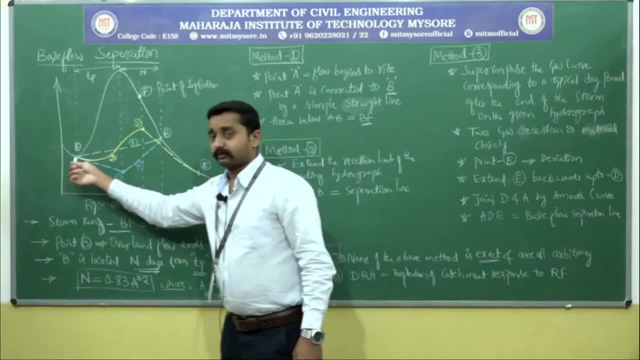 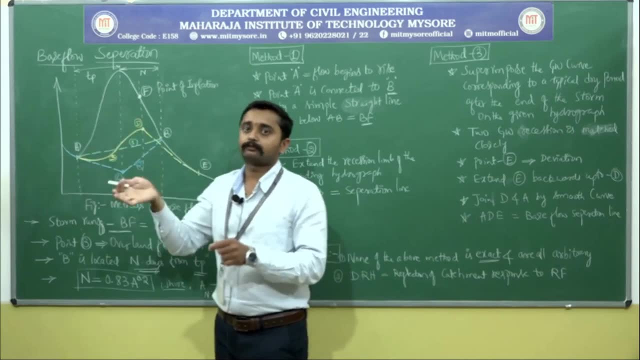 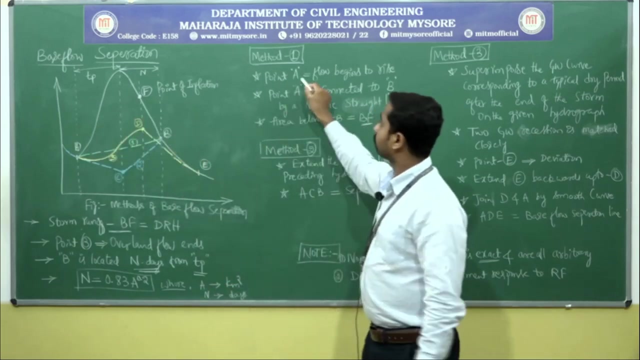 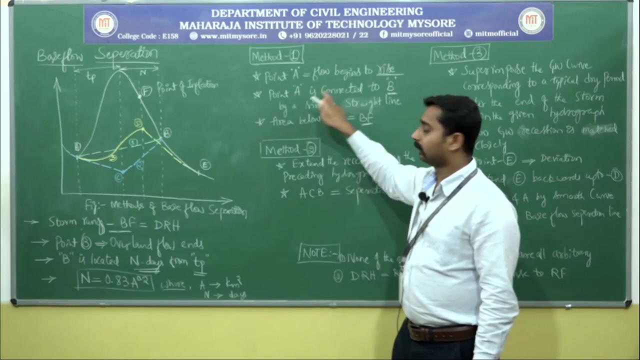 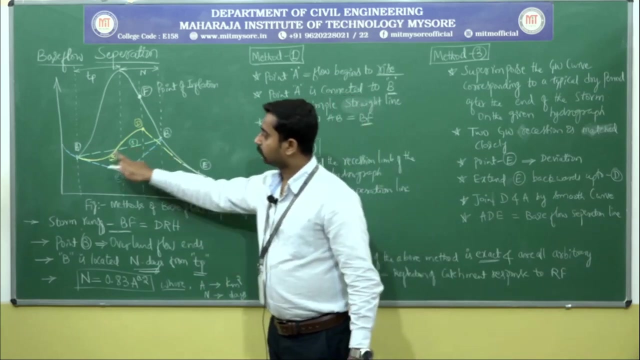 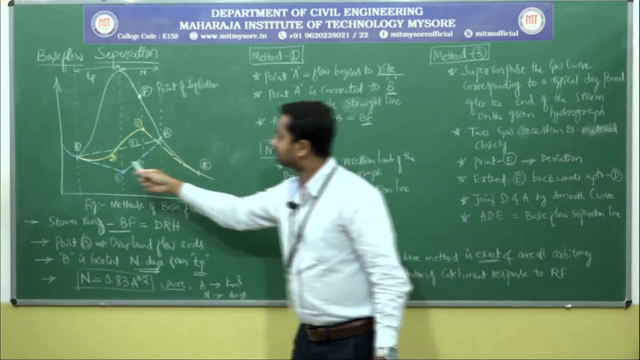 flow began to rise, correct, Alva, Yesterday. only I told you from point A runoff is slowly increasing. After all the losses, runoff is slowly increasing. So point A represents flow begins to rise. Next point A is connected to B. this green color line, Point A, this is point B. Point A is connected to point B by a simple straight line. 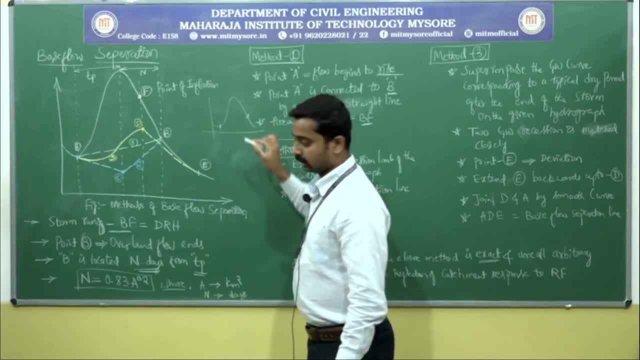 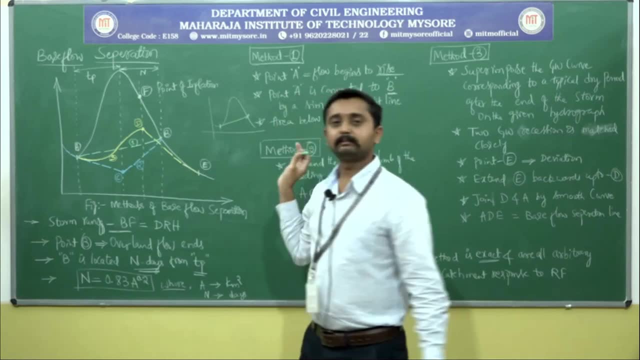 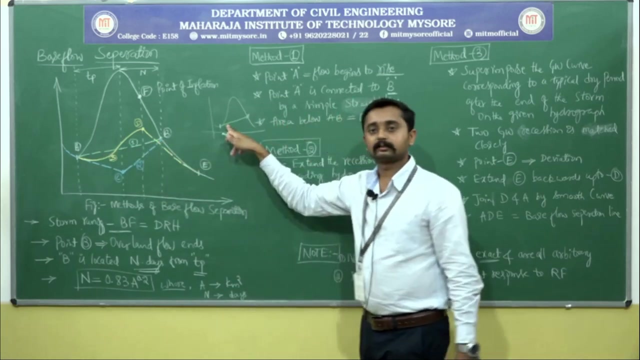 This is point A. this is point B. Just simply connect point A to point B. This is point A. this is point B. Just simply connect point A to point B by a simple straight line. This is green color. this green color: Point A is connected to point B by a simple straight line. 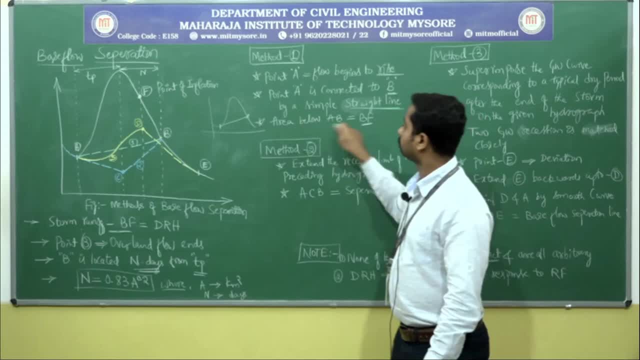 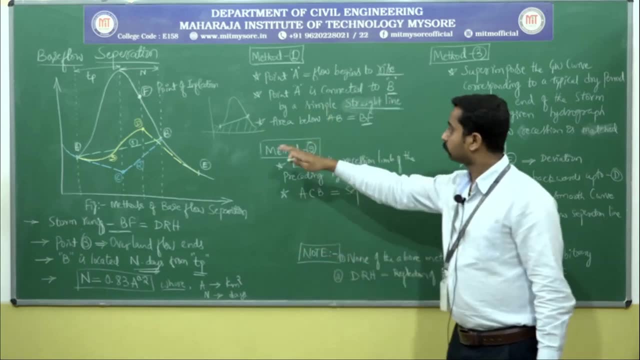 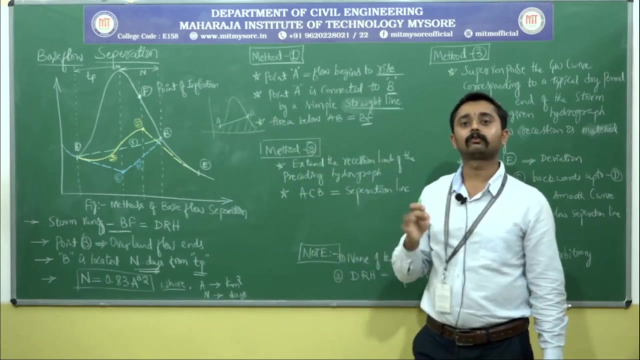 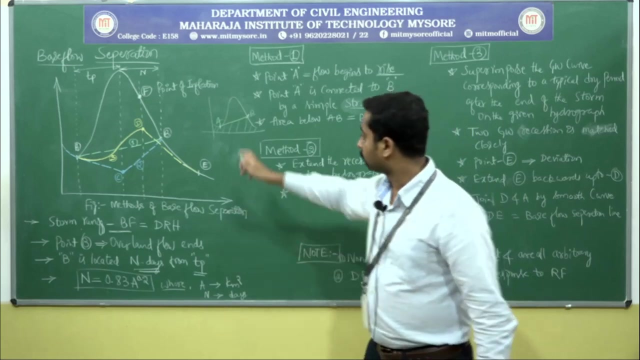 Now, area under this portion, area below this curve, area below this curve, AB below this line, straight line, AB equals to base flows, base flow magnitude, And then AB is a base flow separation line. AB is base flow separation line. 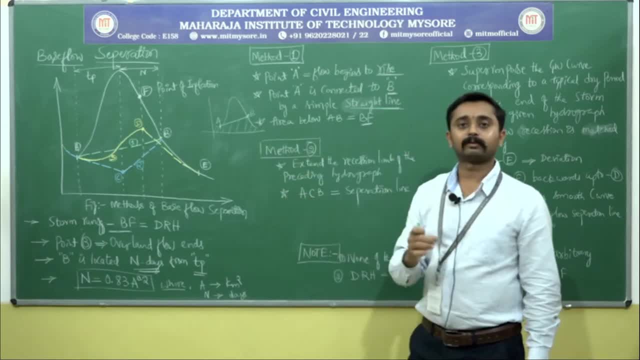 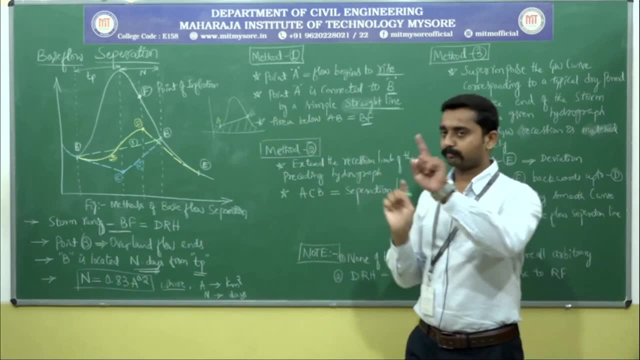 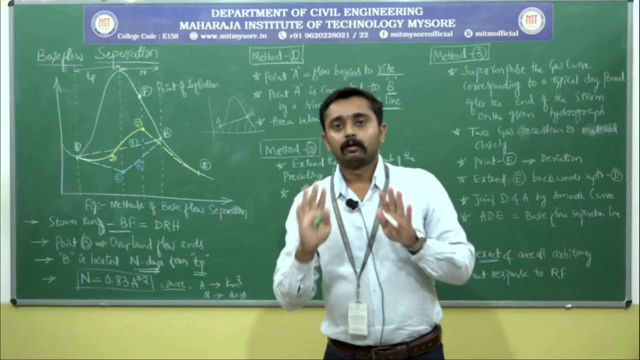 Area under the curve. area below AB represents the base flow quantity. This is very simplest among three: Just point A. point B: just connect by straight line. Area below the curve represents the magnitude quantity of the flow. Area below the curve represents the magnitude quantity of the flow. 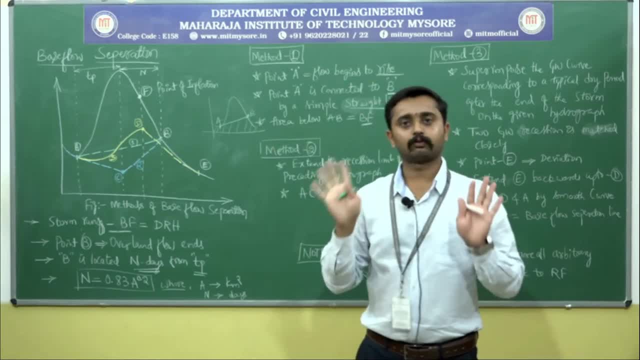 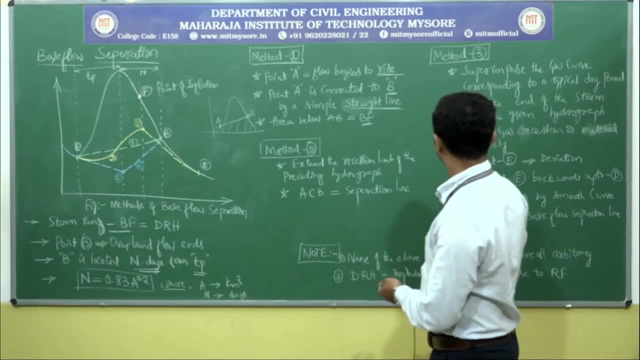 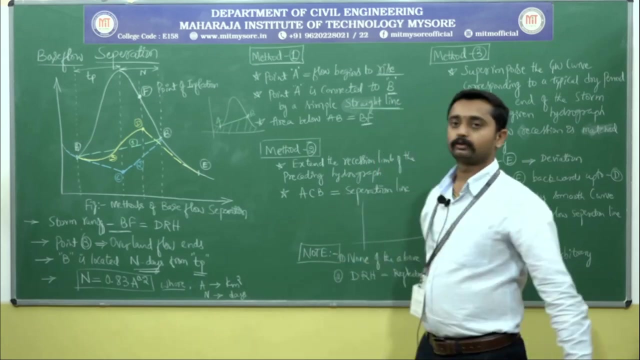 And that line is base flow separation line. Okay, finished. Next method two. Next one is method two. I will write here Method two. Okay, I will write here only Method two. Listen carefully, Method two is represented by blue line. 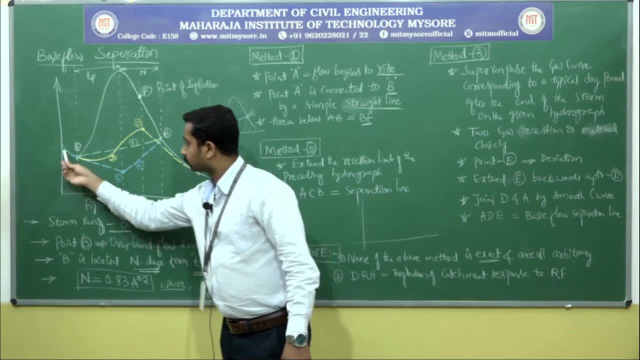 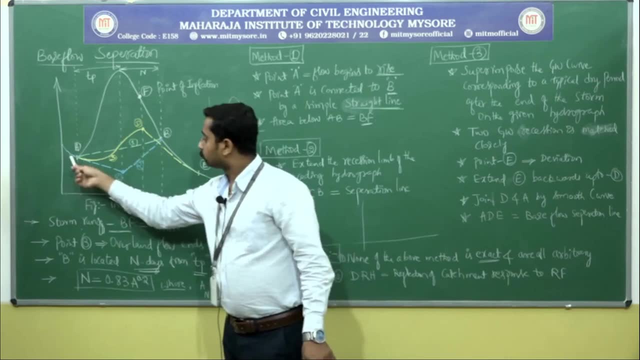 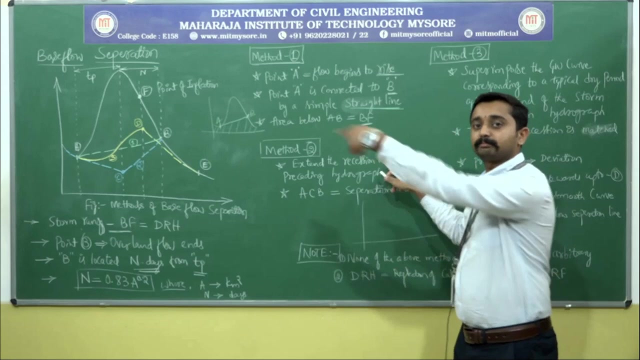 Method two: method two is represented by blue line. Method one is represented by blue line. Method one is represented by green line. That's done. Method two is represented by blue line. Okay, What I am saying is extend the recession, limb of the preceding curve preceding hydrograph. 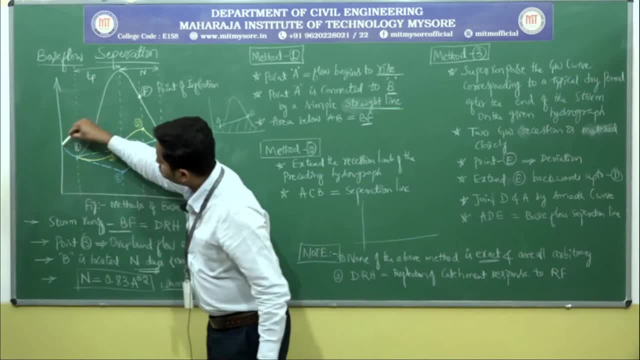 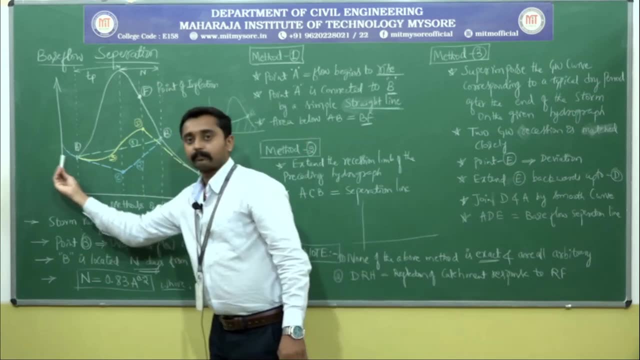 Which one? Listen here. This portion, this is the recession Right. Actually, this is what rising limb, recession limb, This is recession limb, Correct. Let's do this from here. So extend this recession limb of the preceding curve. 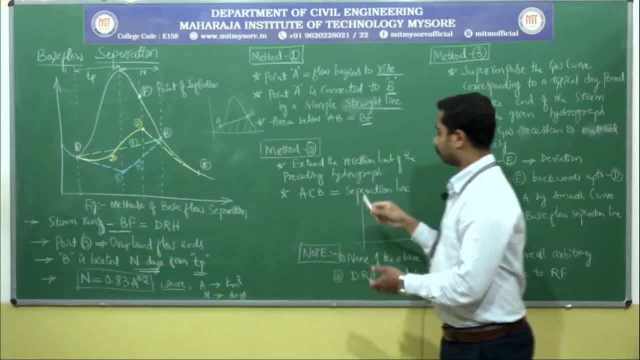 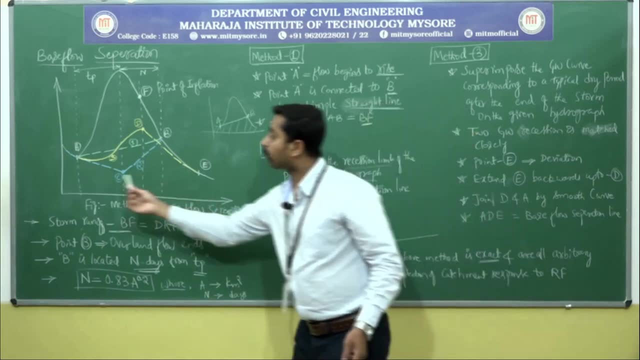 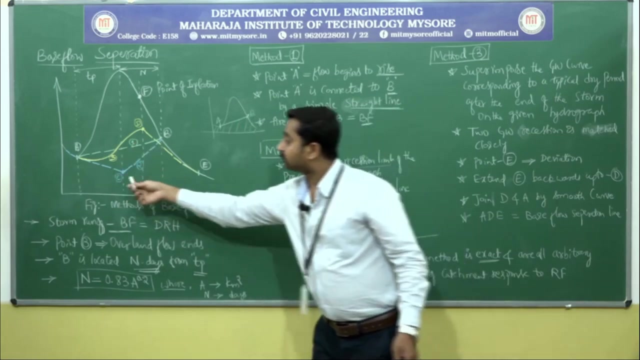 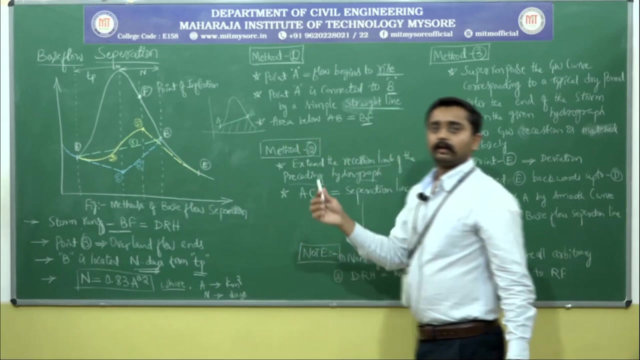 This recession limb of the preceding curve, extend this recession limb of the preceding hydrograph up to point C. up to point C where the point C is on the peak coordinate. The point C just extend the recession curve from point A because just a tangential again. 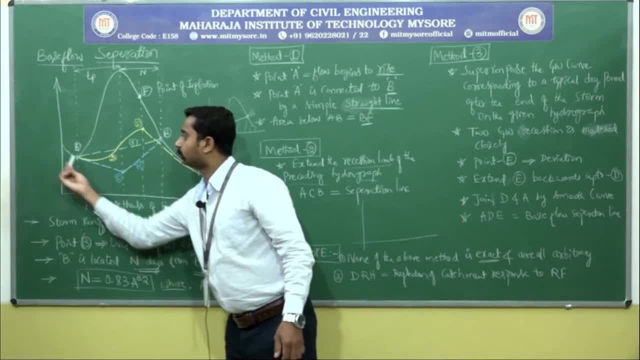 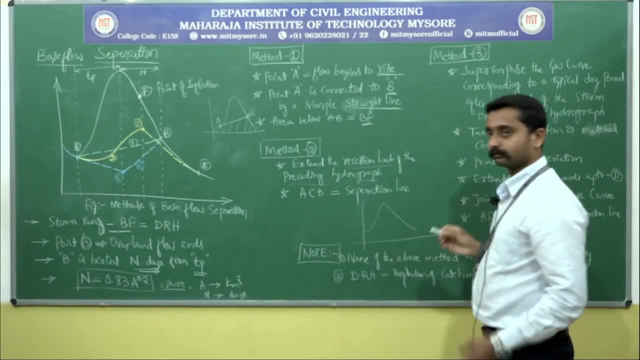 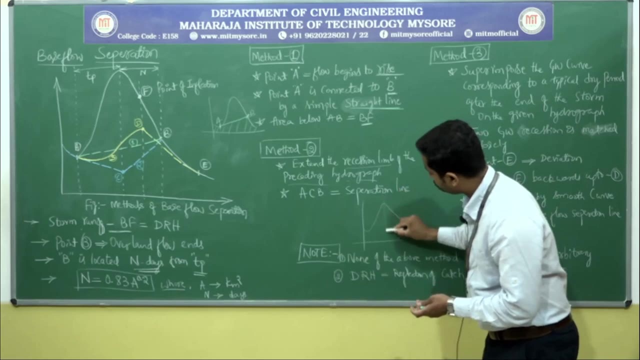 Okay, Just a tangential again. Just a tangent to point A. It is done. Actually, the hydrograph is like this: This is the hydrograph From here. this is the peak coordinate, Correct, This is the peak coordinate. 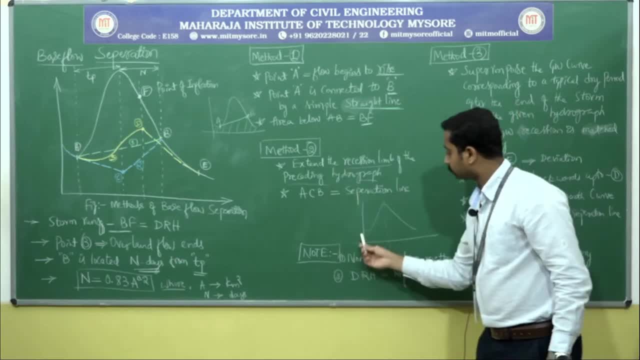 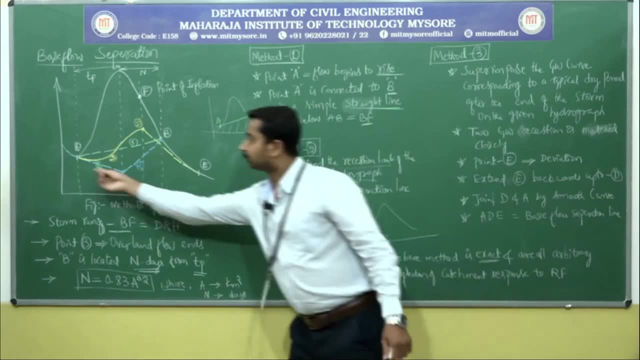 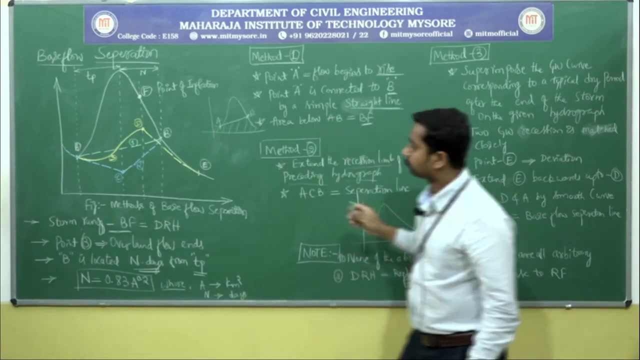 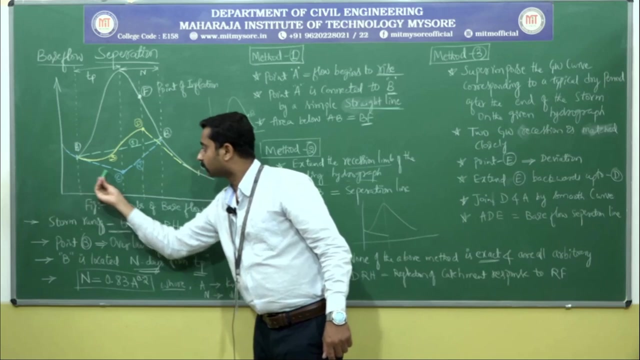 This is the peak coordinate. Extend this recession limb of the preceding curve up to this point. Just a tangential to this line. line, just tangential to the recession small recession portion. This is very small, This is a small recession portion. Tangent again, just extend this line. just extend this line up to 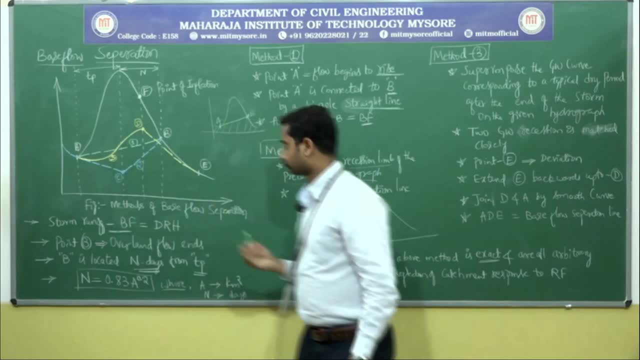 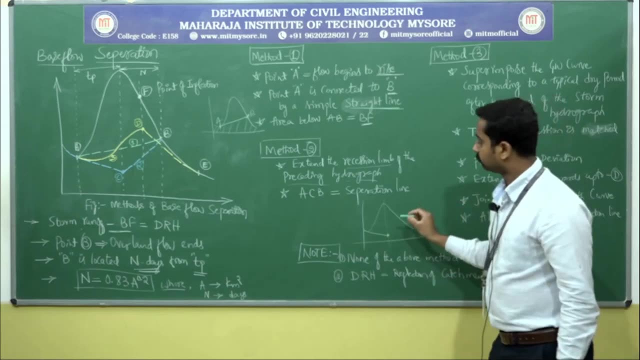 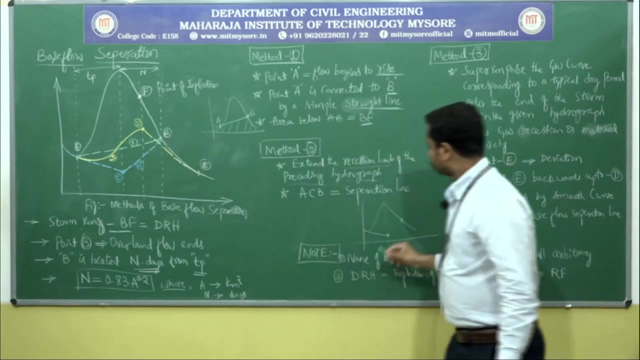 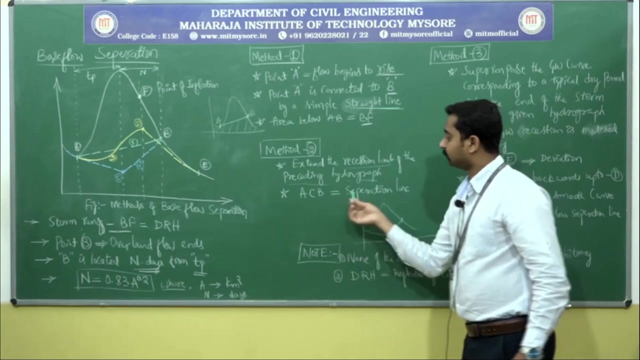 point C. Point C is on the peak coordinate. Point C is on the peak coordinate. You will get this point Now. it is very simple. Just connect this point C point to B. point B point is already there. Just connect this point by a straight line. Now, area under ACB. this is the point A. 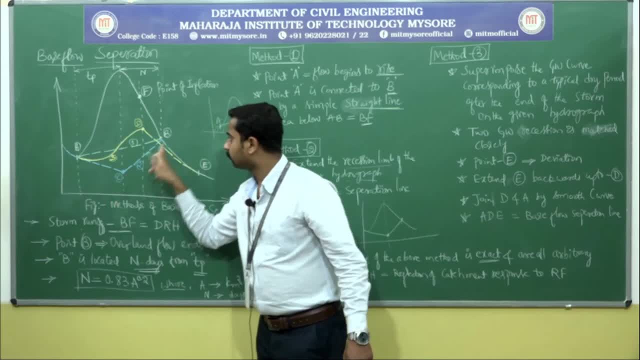 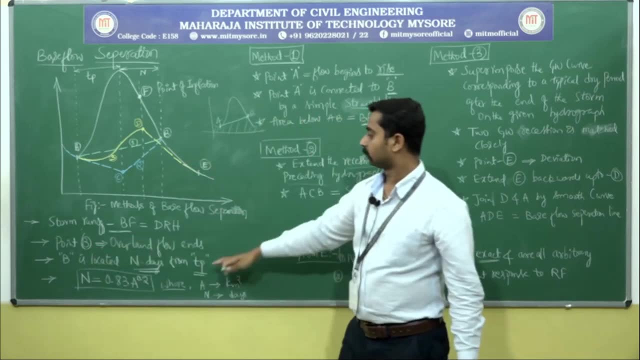 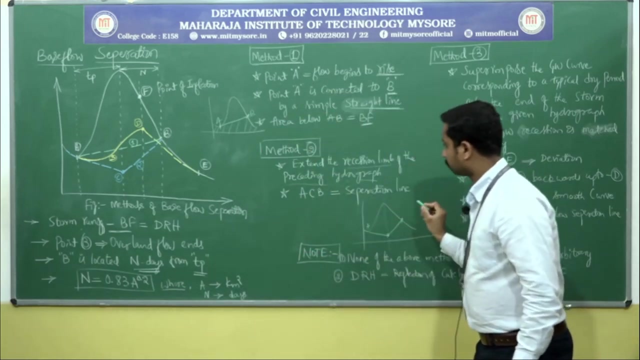 Listen carefully. This is point A. This is point C. This is point B. I said already how to locate point B. So from end is B is located, end is from peak coordinate. Now, this is point A. This is point B. We know Now. 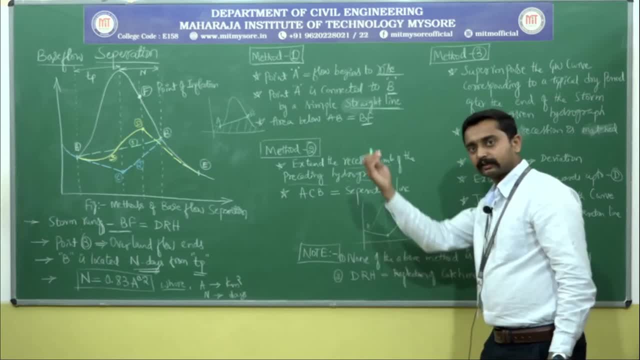 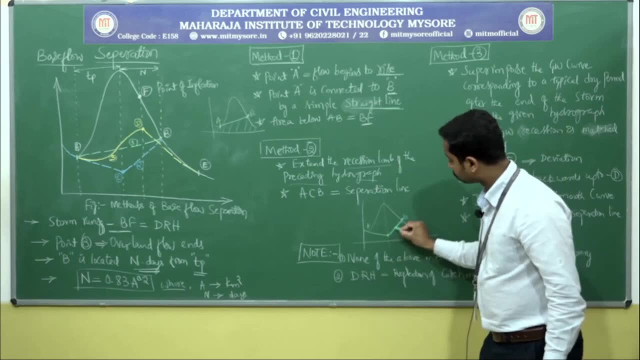 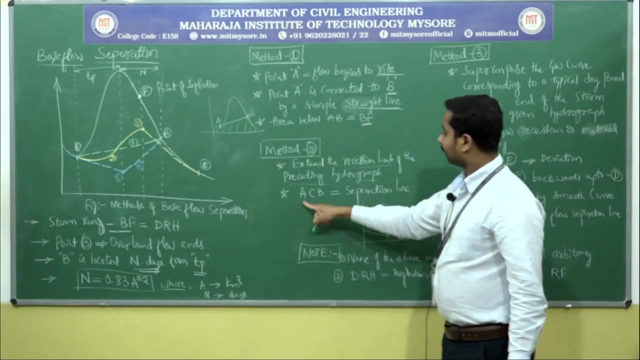 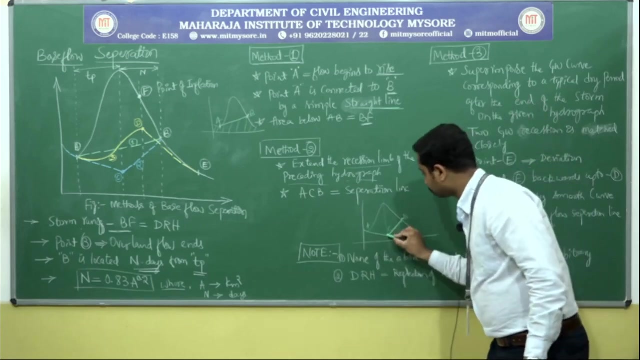 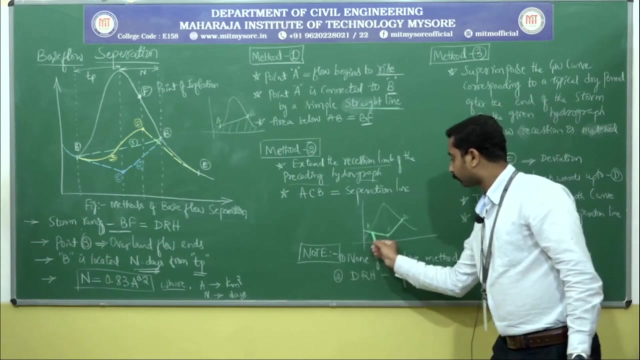 we just extended this line tangential to the recession limb corresponding to this peak coordinate. After that, just join this line. Just join C to B. Now ACB, A, C, B. Now you can connect with C here. Go back to your first line and add it. I have taken some. 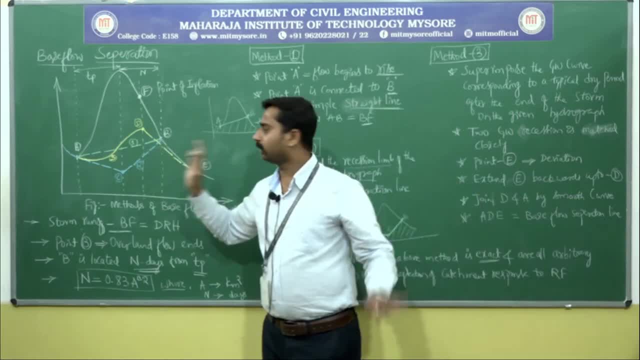 song now. So this B and ACBever, See for your B. actually it would be same like this, And this line will be the earlier line. Now, from these three lines we just need今日. and the second line is B point Now. now, if I move on. so rails to the peak coordinate. 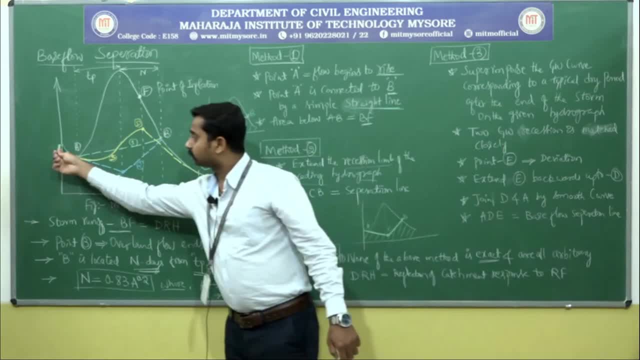 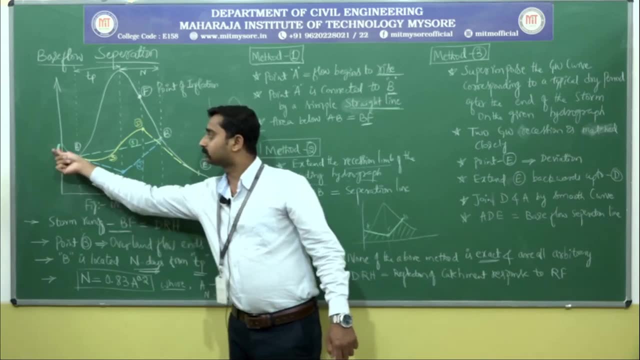 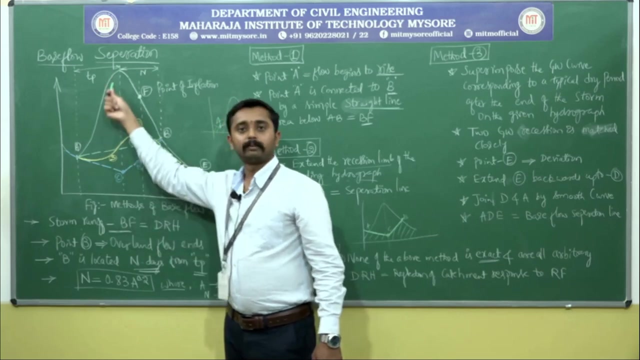 We cannot do this further. Only the former line can join with this. Look for the region of this line to. we just extended the recession portion in such a way that just tangential, just a tangential, to this recession portion up to point C, and the point C is on this line P. 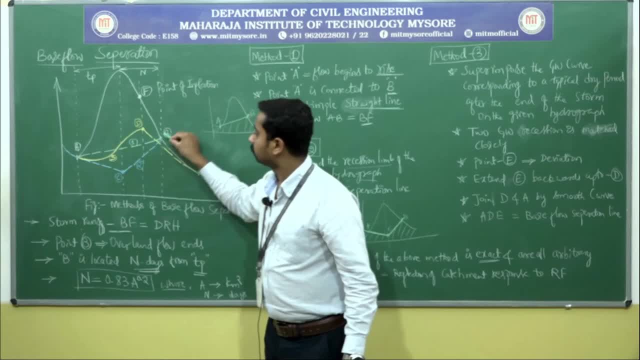 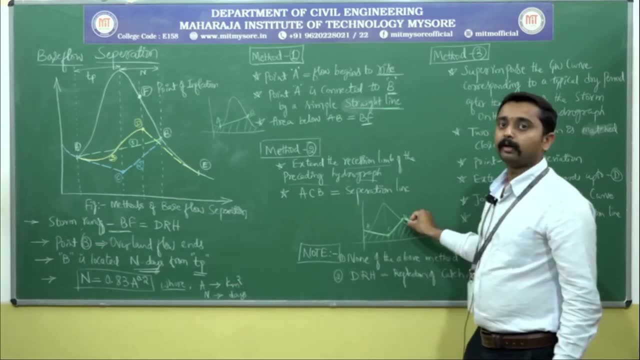 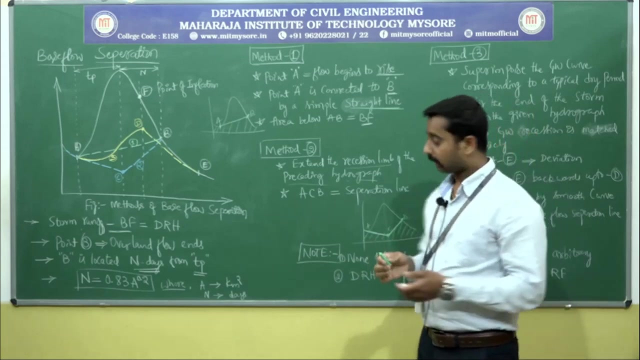 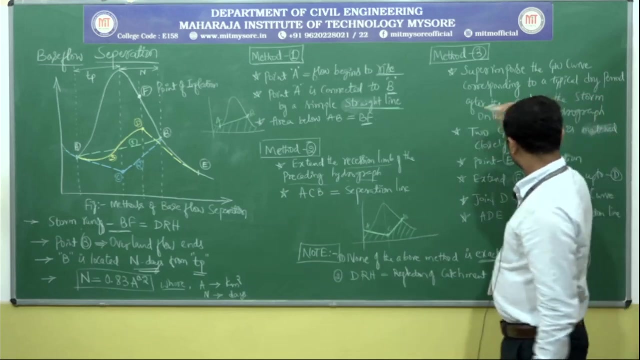 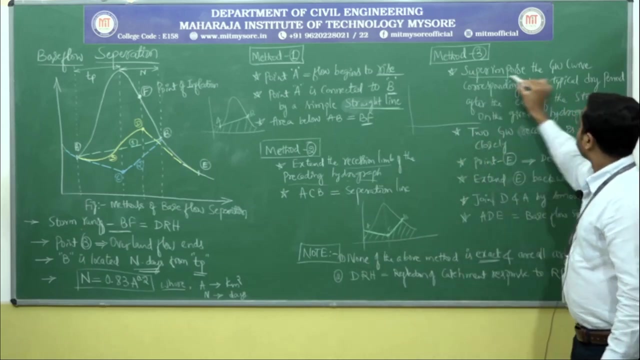 coordinate. After that just join C to B by a simple straight line and this ACB represents base flow, separation line and area under the curve ACB represents quantity of the base flow. And third method. last one is third method. listen now I will write here: superimpose. 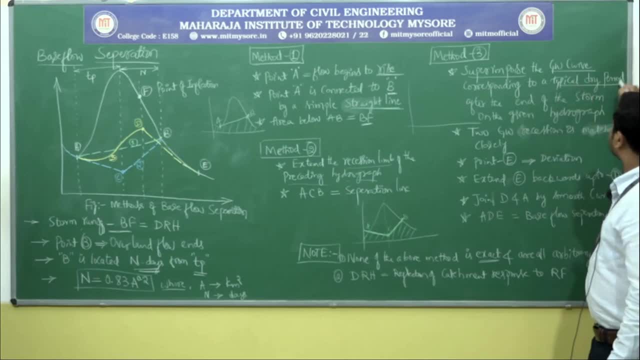 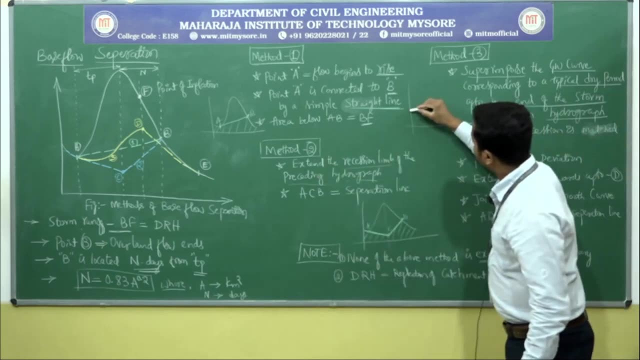 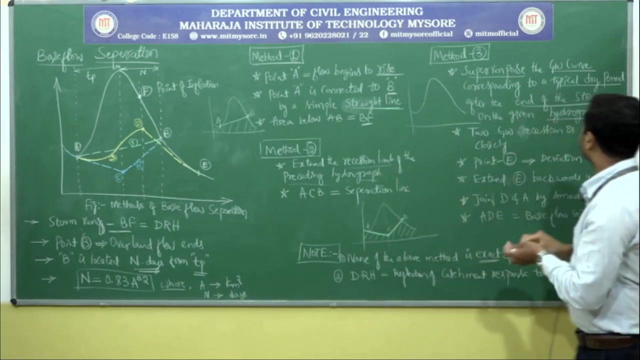 the ground water curve corresponding to a typical dry period after the end of the storm. on the given hydrograph. That means already there is a hydrograph. this is the hydrograph. on this hydrograph, only just to superimpose, just superimpose the ground water curve corresponding to the 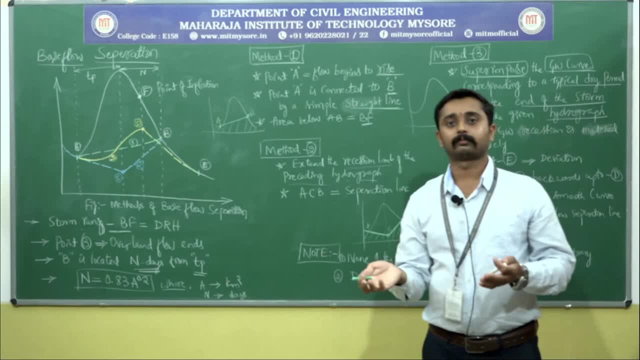 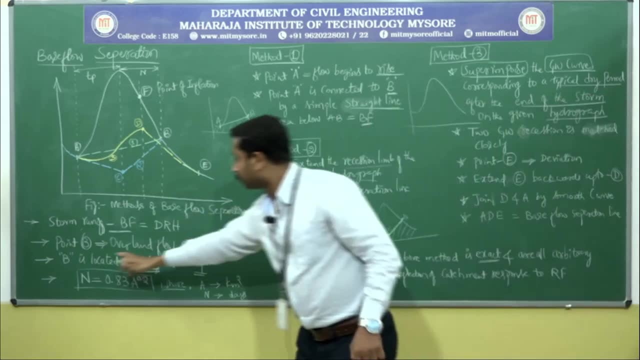 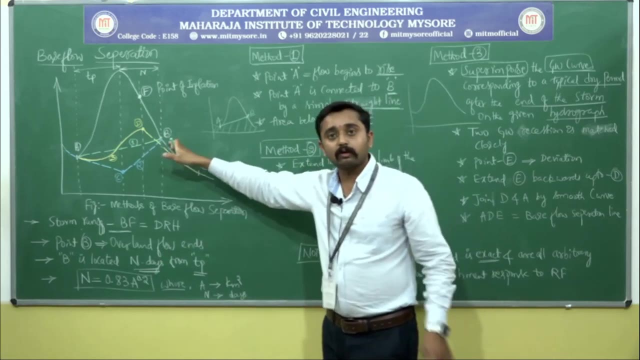 dry period: typical dry period after the end of the storm. storm end base flow should be like this: See, just I said point B, nothing but over land flow. That means point B represent end of the over land flow. over land flow is created here. 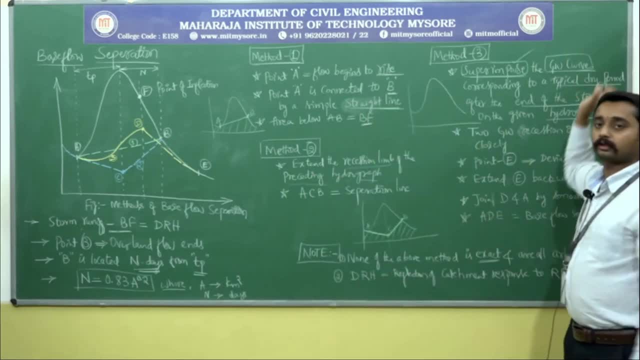 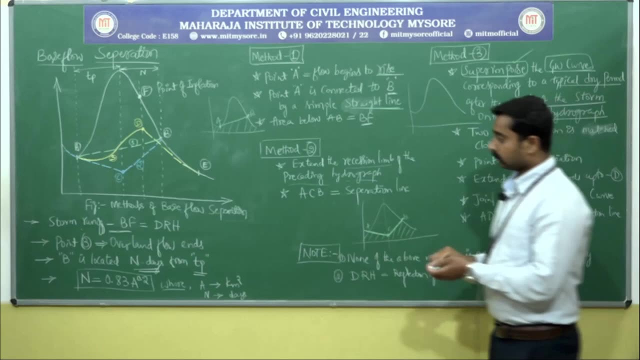 base flow should be like this. So now what I am doing is just to superimpose the ground water curve on the same hydrograph. just superimpose the ground water curve on the same hydrograph. okay, again it has come. 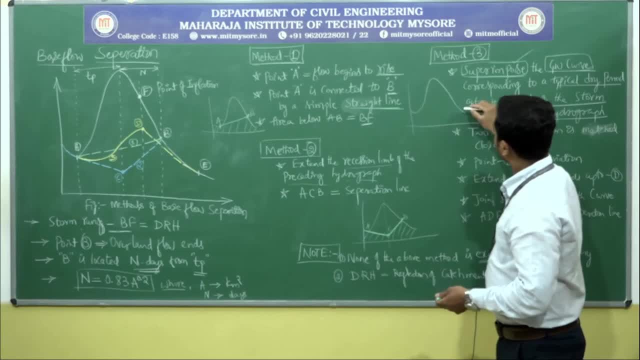 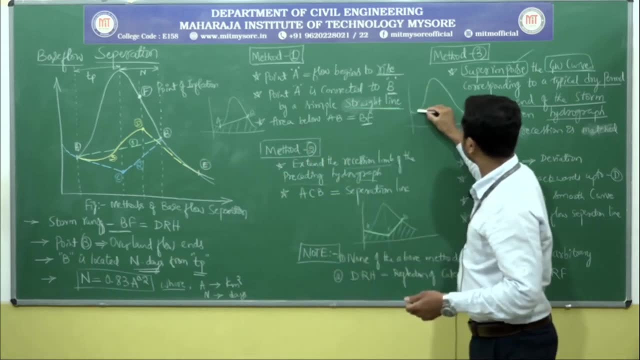 here almost you will get like this, only There is some little deviation. okay, like this: there is some little deviation. on this same curve there is another ground water curve, So there is some little deviation. like this: There is some little deviation. 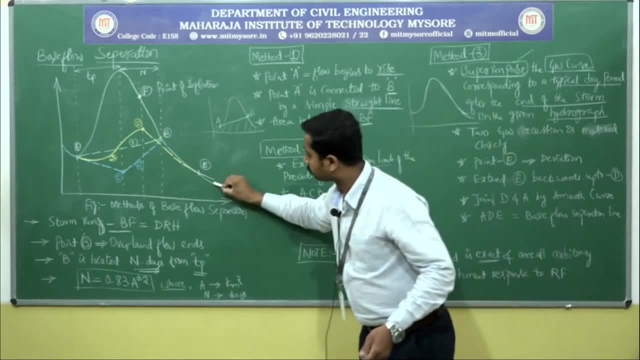 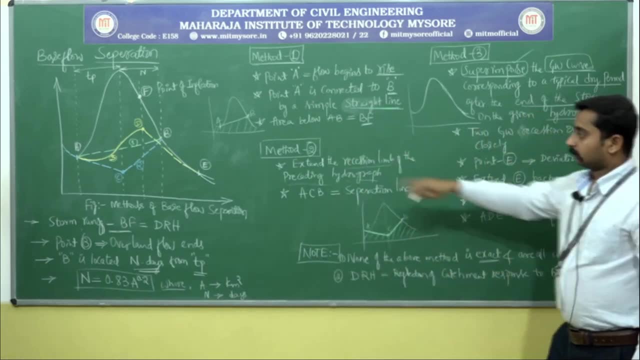 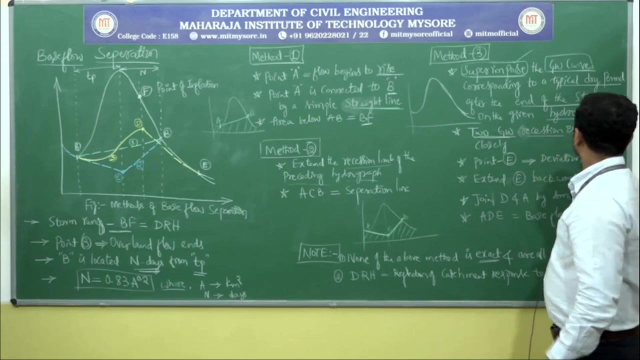 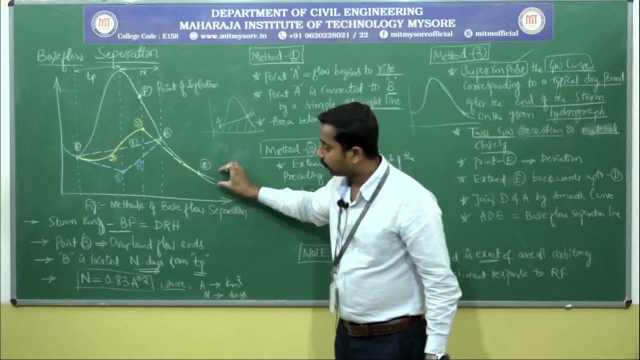 So what I am doing is I am drawing a small deviation. okay, this is the small deviation, just superimpose. okay, now there are two curves here. be careful. two ground water flow recession is matched closely listen. two ground water flow curves matched very. 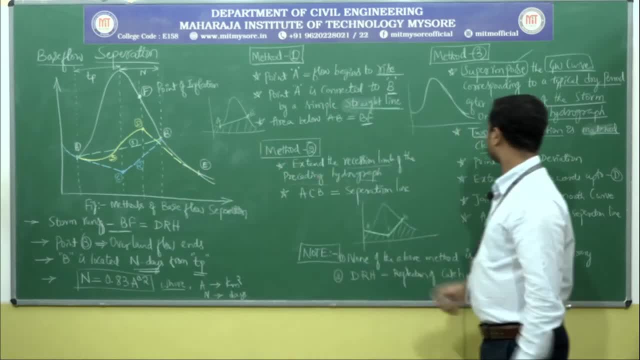 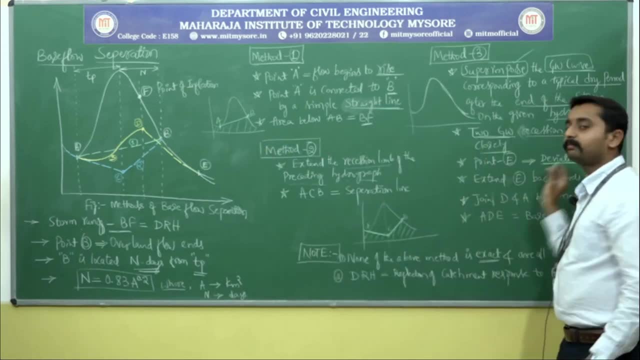 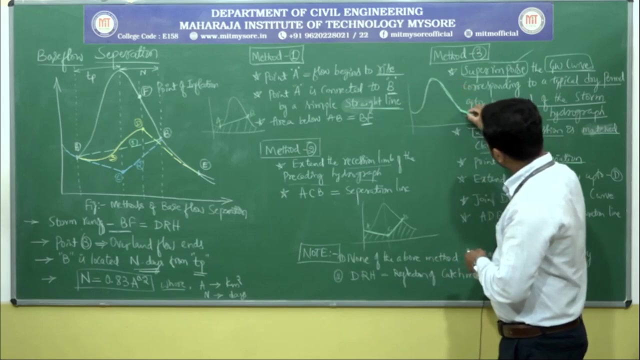 closely. draw carefully. almost it will be like this: draw carefully The point E, this, this point E takes some deviation, okay, and then here I will just call it green color. see when point E comes. this is the first. hydrograph is this, and 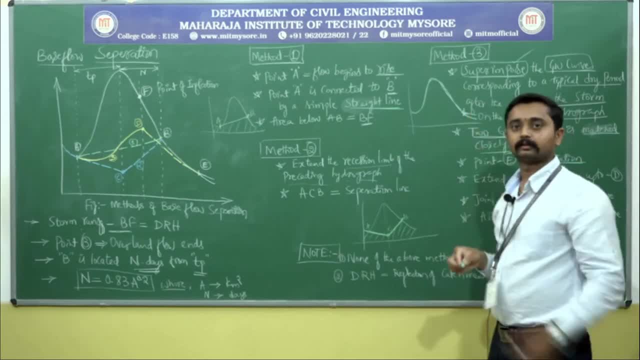 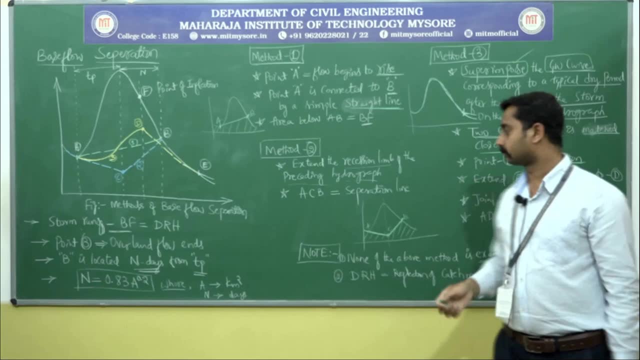 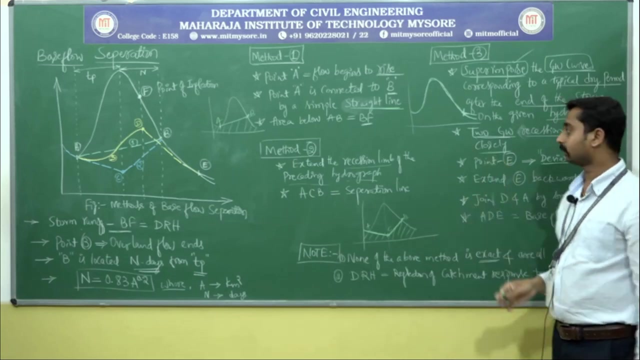 now, the second hydrograph is this. So this is the point E, the point E where it has to be located. the curve just takes a deviation. okay, Point E. locate just that, take the deviation. locate that point as E. Now extend this point. 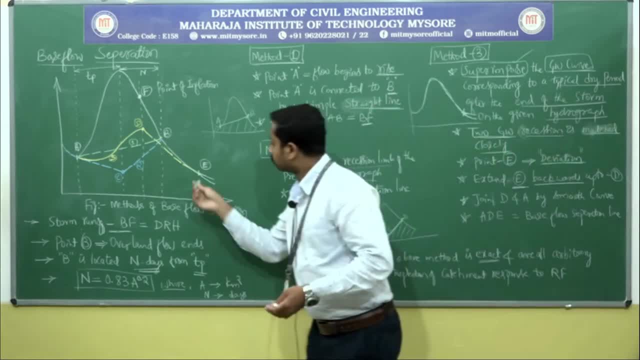 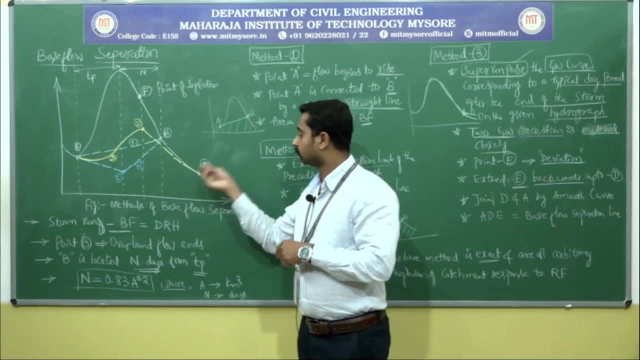 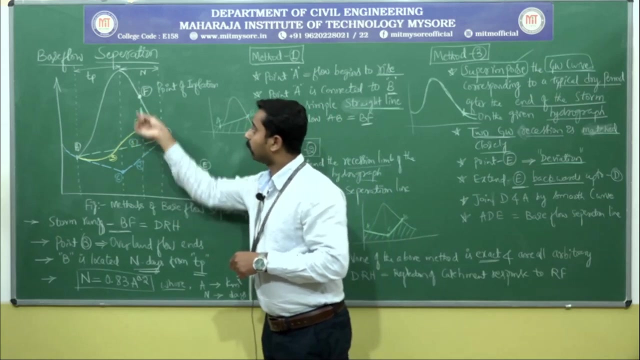 E backward up to D. you will notice, extend this curve, just deviation. just mark it as E, just mark it as E. Now, extend this backward, extend this curve backward up to point D. that point D is on point of inflection. 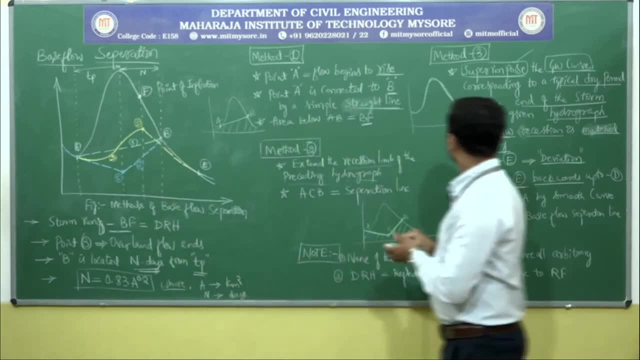 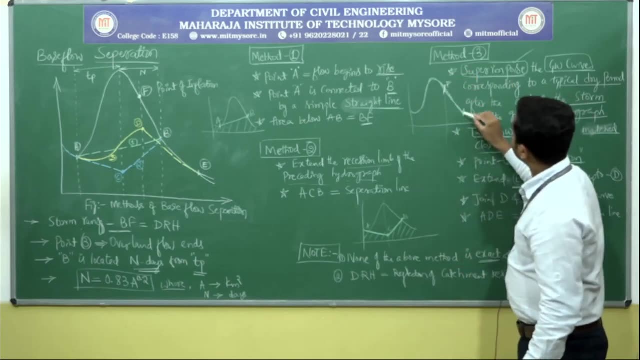 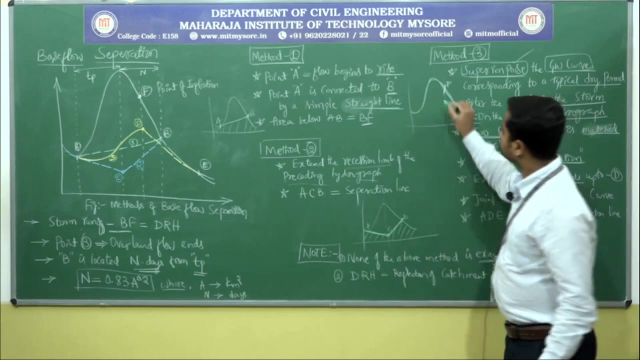 Okay, Okay. So this is the point of inflection F. just, this is the point of inflection F. okay, just extend this line backward, just extend this line backward, so cut it. so this is the point D, okay. 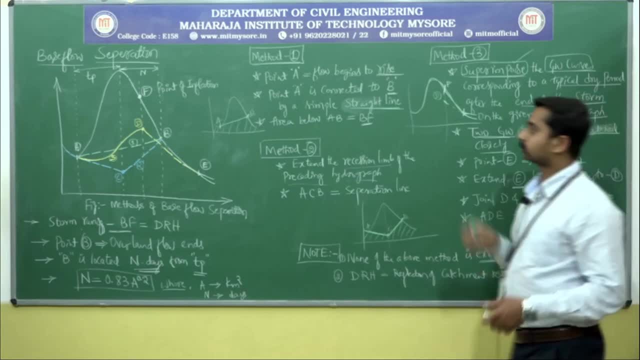 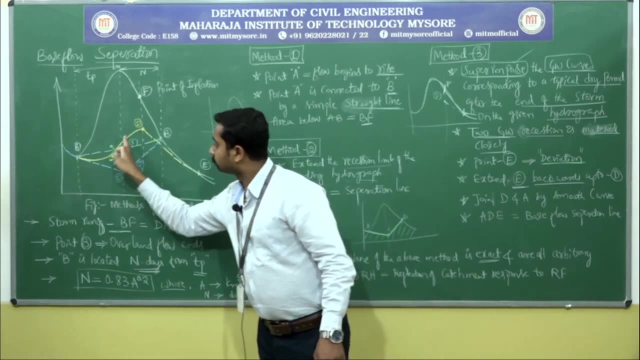 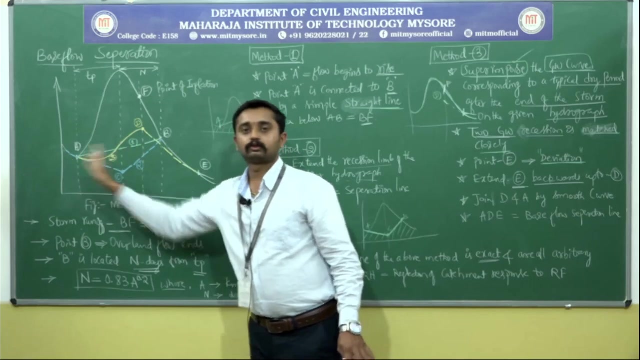 Now join D and A by a smooth line. so this is the point. D same point. just join D and A by a simple line. Join D and A by a simple approximate smooth curve. join D to A by a simple approximate smooth curve. okay, smooth curve. 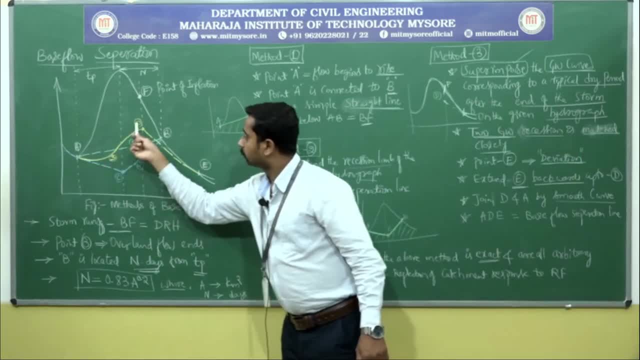 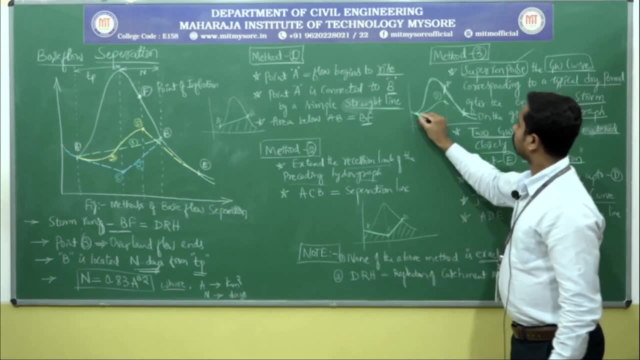 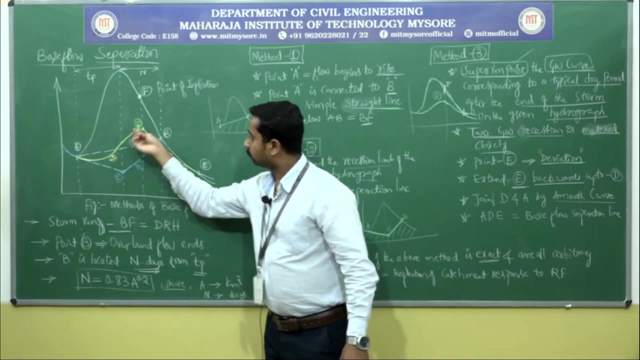 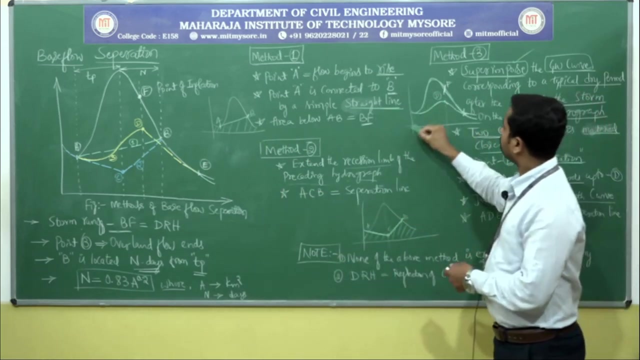 Now, ADE, ADE. this one, this one, ADE. the line represented by yellow ADE. the line represented by yellow ADE, ADE, ADE. Now, this is the base flow separation line and area under this curve represents the. 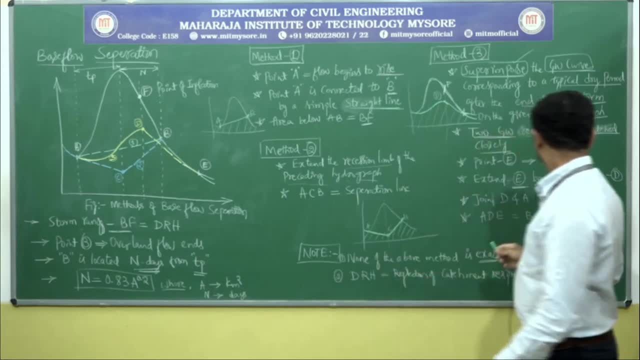 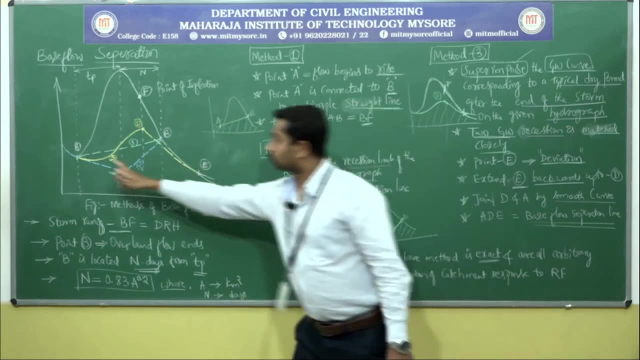 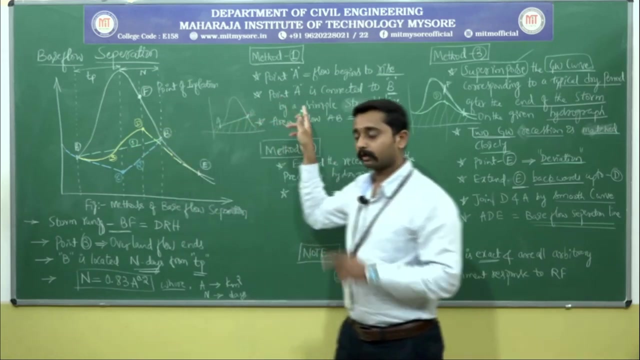 magnitude of the base flow. okay, This is all about base flow separation In the first method. just join AB by straight line. just join AB by straight line. green color: the line represented by green color is the base flow separation line by method. 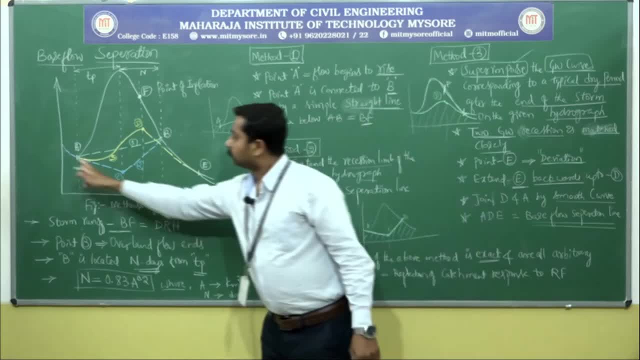 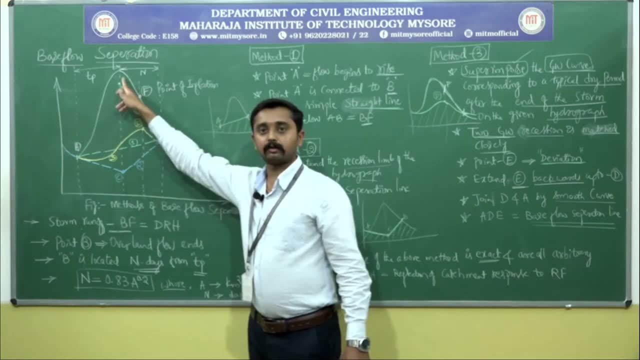 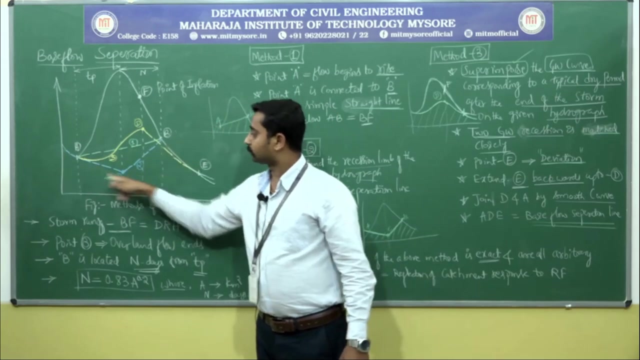 1. Second method: just this recession limb. extend this recession limb up to the point C. the point C is on the p coordinate. then join C to B by simple straight line. you will get A- C- B. the line represented by blue color is the base flow separation line by the second. 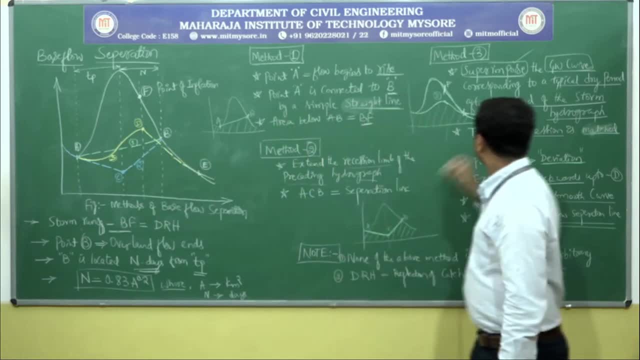 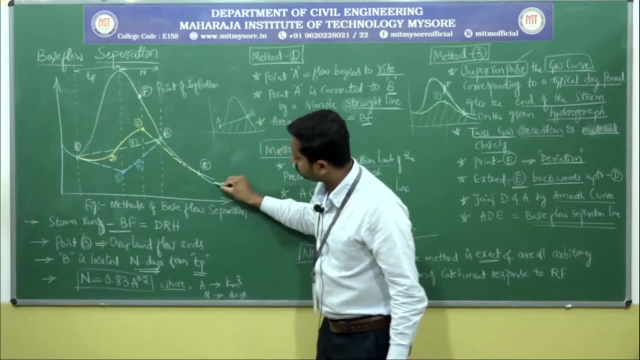 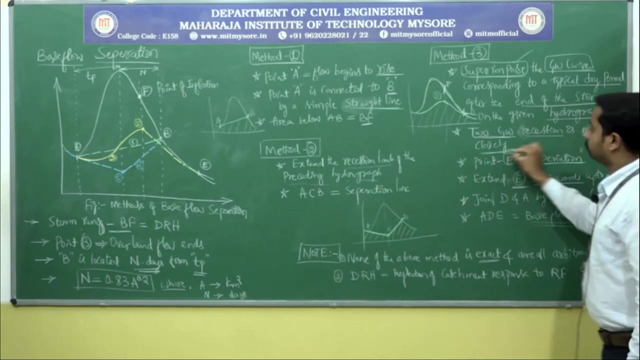 method. and third method: just superimpose groundwater flow curve, superimpose railway abord waqf, superimpose the groundwater flow curve, State 되게. That takes some deviation here, little deviation that match closely, match closely, two ground. 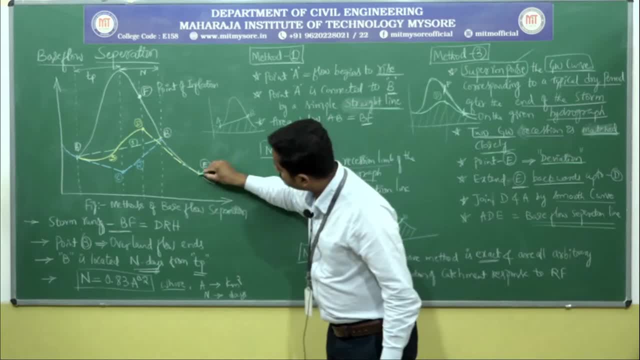 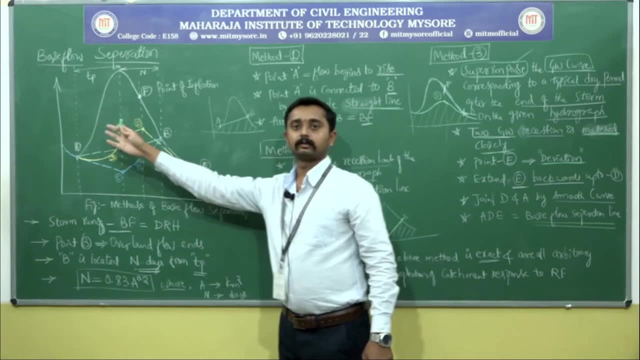 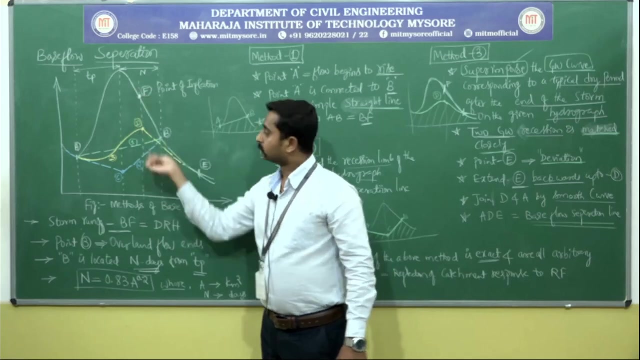 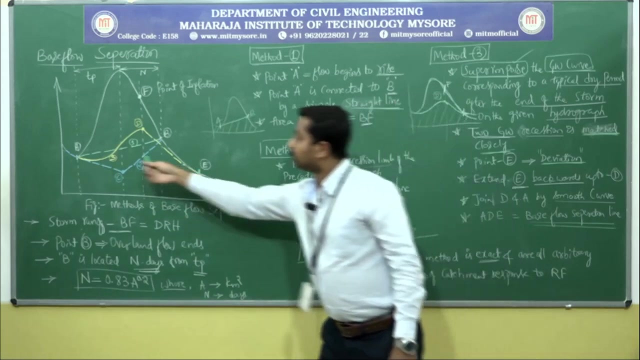 water flow curves are matched very closely and the deviation the two curve takes deviation from here. mark that point as E. just extend backward, just extend backward up to the point D. the point D is on point of inflection. Now just join D to A by simple approximate smooth curve. now the line represented by 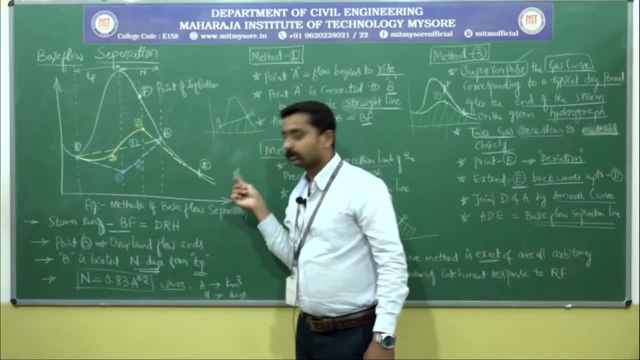 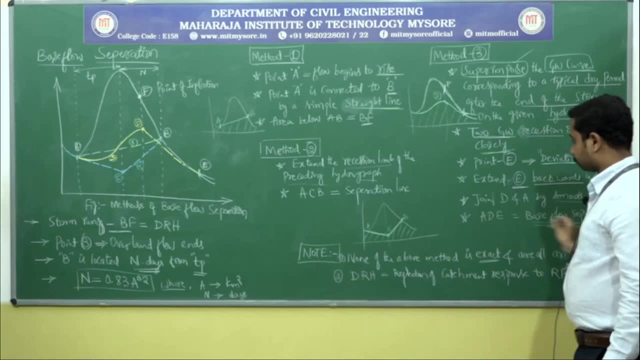 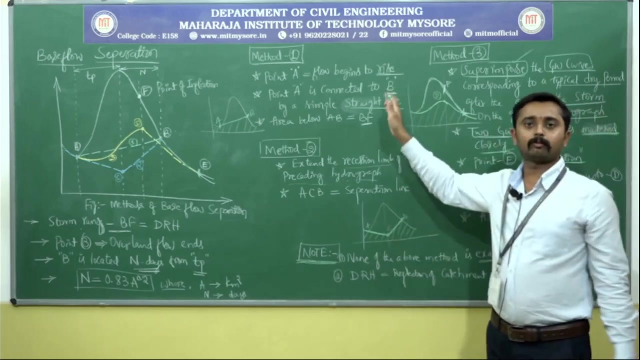 yellow color: A, D, E is the base flow separation. line area under that curve represents the quantity of the base flow. This is all about base flow separation and this point is very important. note: you know none of the above methods. none of above: method 1,, method 2,, method 3.. 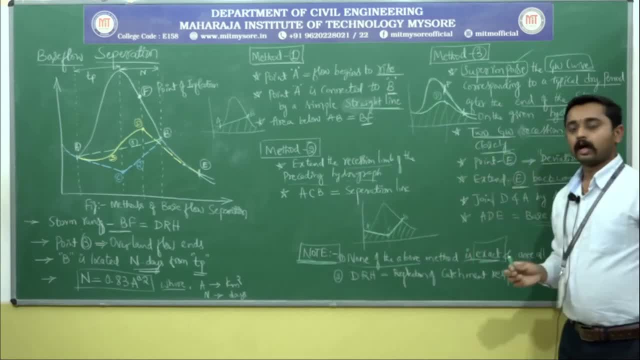 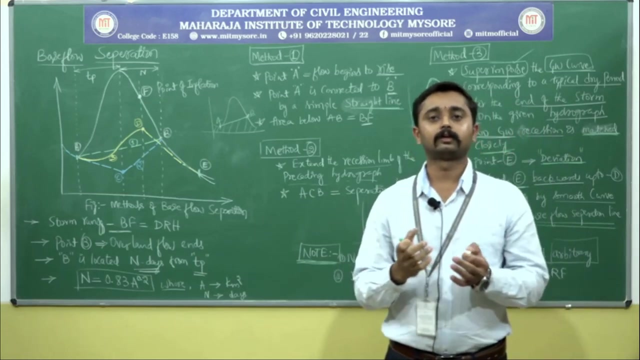 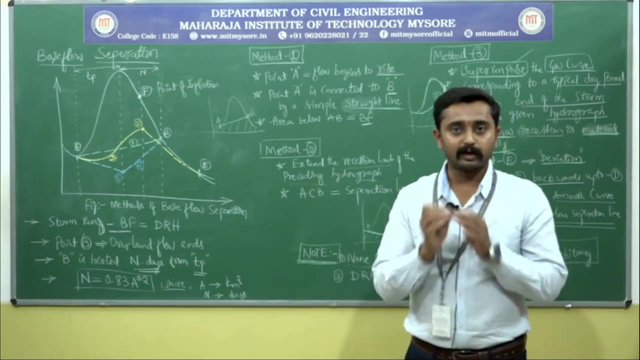 None of the above methods are exact and they are all arbitrary. none of the methods are 100% correct. Why is this? And there is no much significance. greater significance to the base flow, I told you in the previous session, only base flow magnitude is very small, and that too. 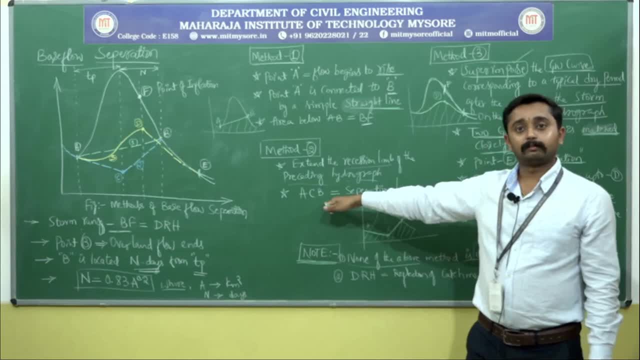 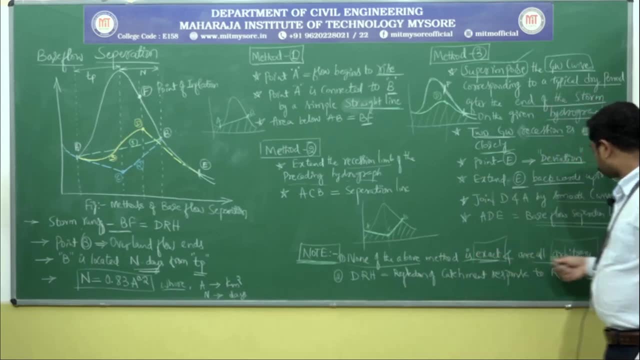 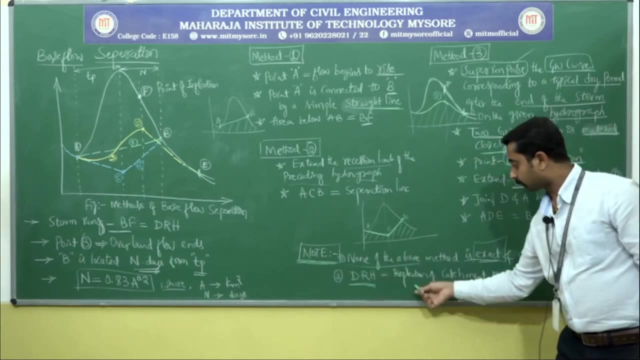 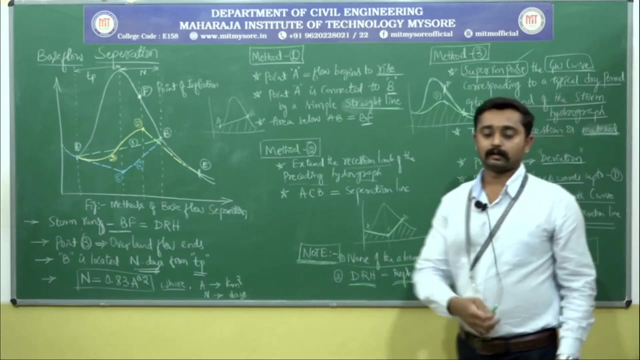 that takes years together. So that's the reason, While preparing hydrograph, we must separate the base flow. base flow, arbitrary, and now the thing is, direct runoff hydrograph is nothing but that represents the that reflect the true catchment response to the rainfall. and there, after the separation of the base flow, 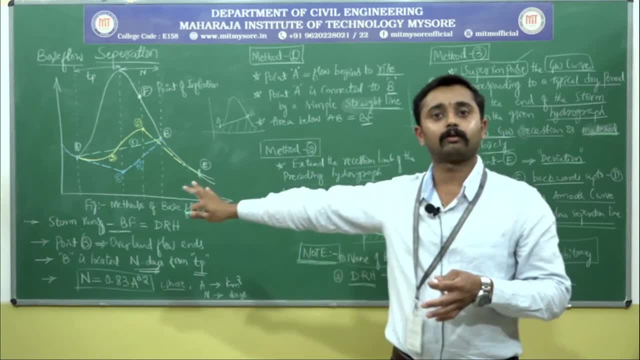 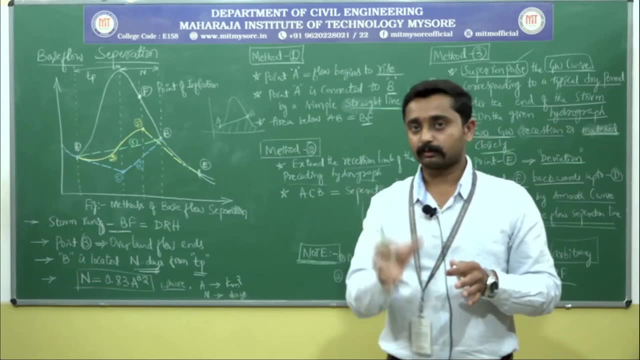 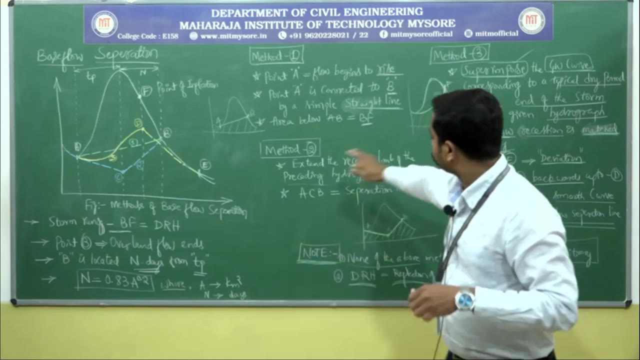 much care is needed. base flow separation is very important because the magnitude is very less And that, too, takes too much of time. In order to prepare the hydrograph, we need to separate the base flow, because the major reason is the magnitude is very low and that takes too much of time. 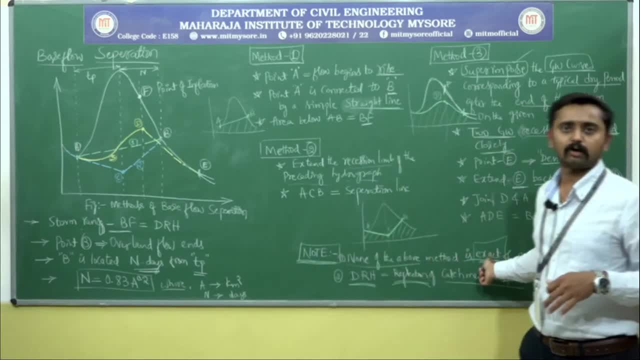 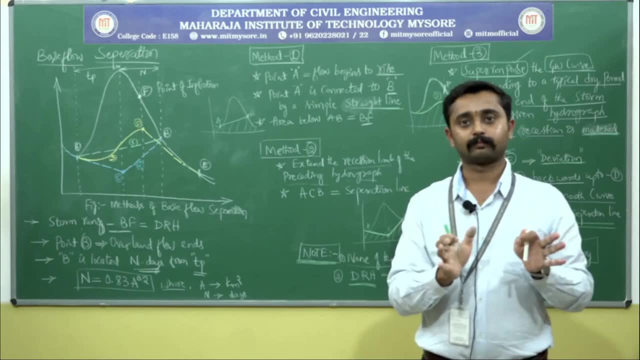 Up to this point because none of the methods are exact. none of the methods are 100% exact, but somehow we need to do the things, because magnitude is there but less magnitude is there. So, after separating the base flow, much care is needed After separating the base flow. 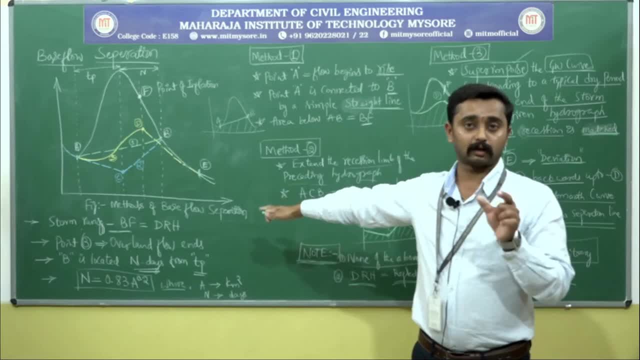 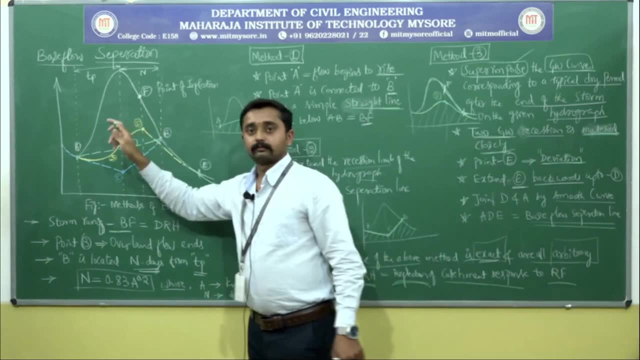 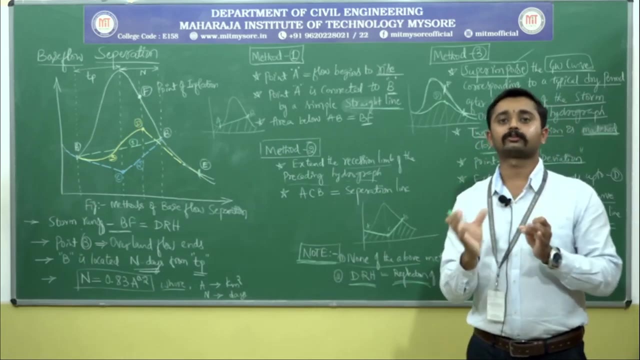 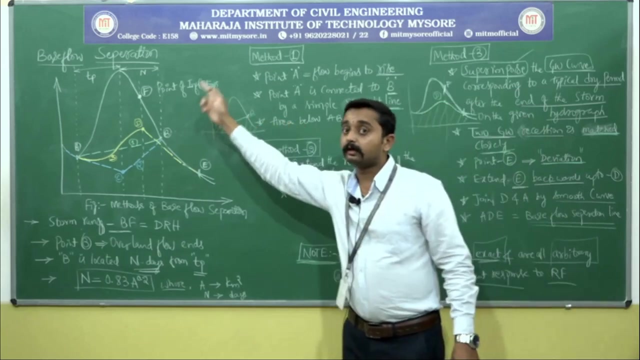 We need to do the analysis with much care and attention, because direct runoff hydrograph, this white line, direct runoff hydrograph, what is there That represents the true catchment response to the rainfall? because if the base flow is very slow, the catchment response directly depends on direct runoff hydrograph. 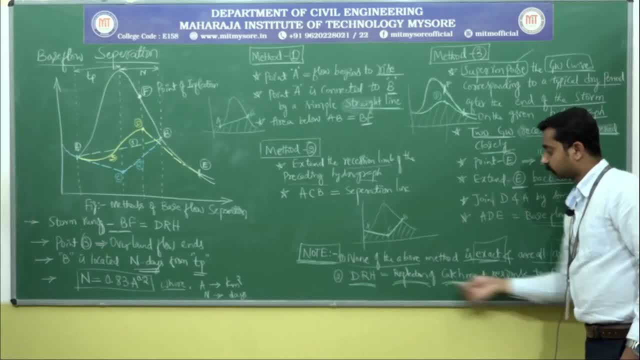 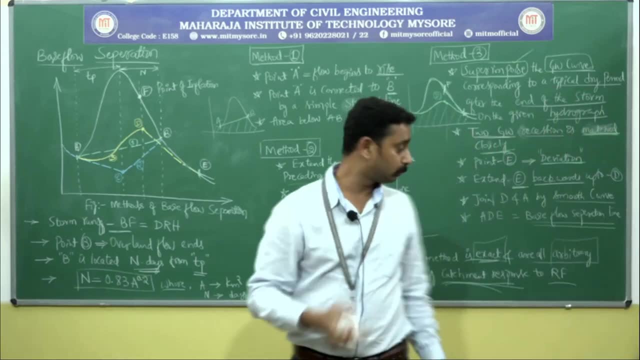 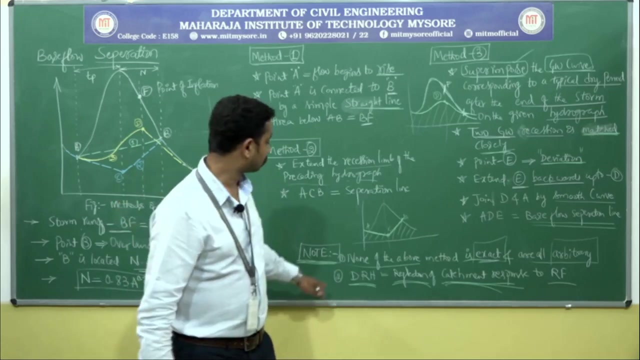 Okay, That is the true catchment response. This direct runoff hydrograph represents true catchment response to the rainfall. Okay, These two notes are very important. One is: none of the above methods are exact. Okay, Somehow we need to do. 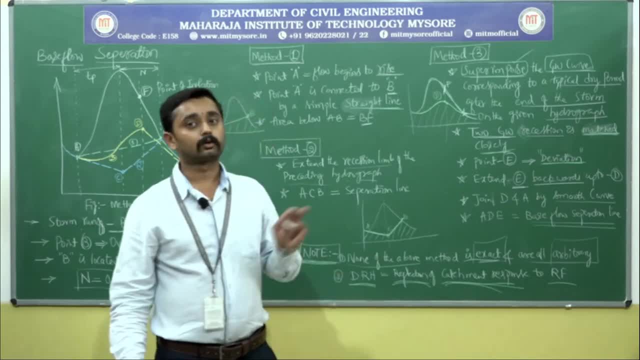 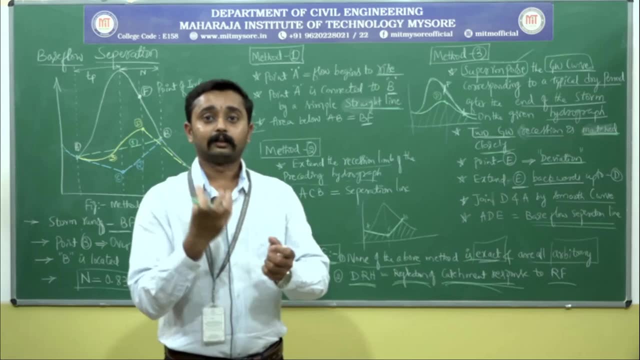 And third. one second point is direct runoff hydrograph is the true representation of the catchment response to the rainfall. Rainfall is important because the catchment response depends on the rainfall. Not all rainfall runs off. Please remember Part of the rainfall infiltrate 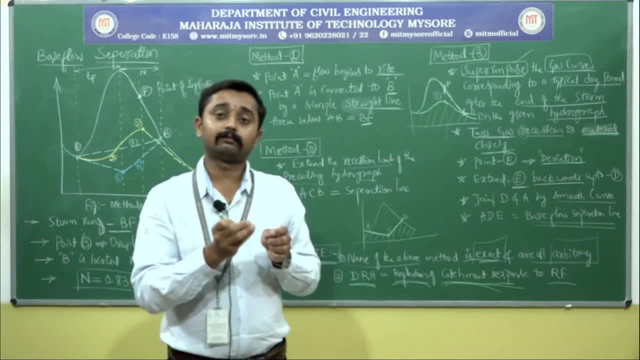 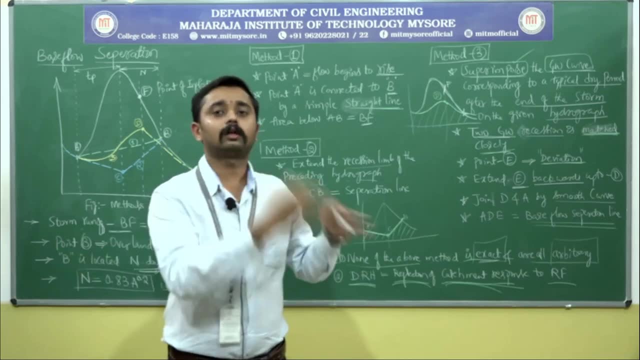 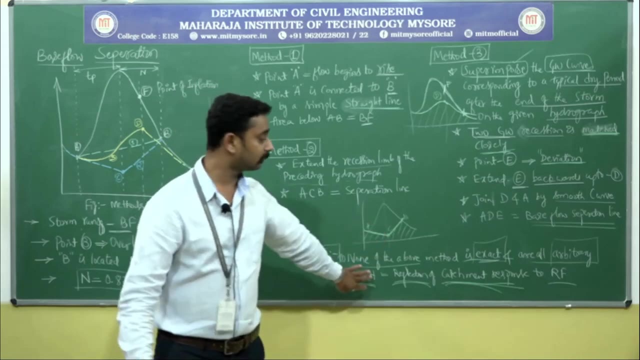 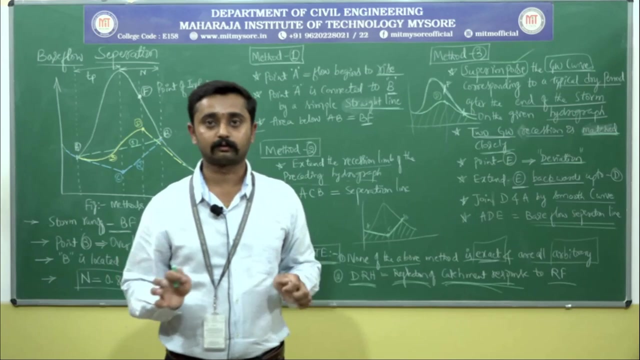 Part of the rainfall inter flows, Part evaporation, And part of the rainfall is the depressional storage. After all the losses, only we get runoff. So that is the reason why this direct runoff hydrograph represents the true catchment response to the rainfall. 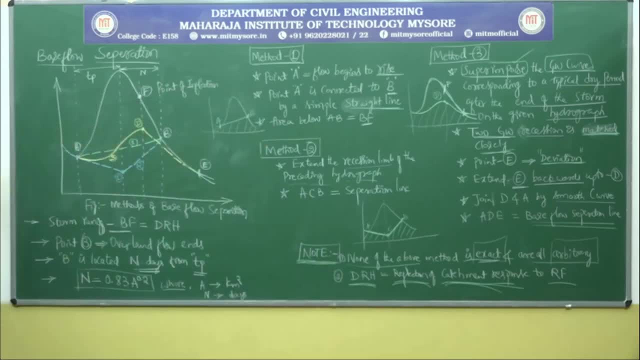 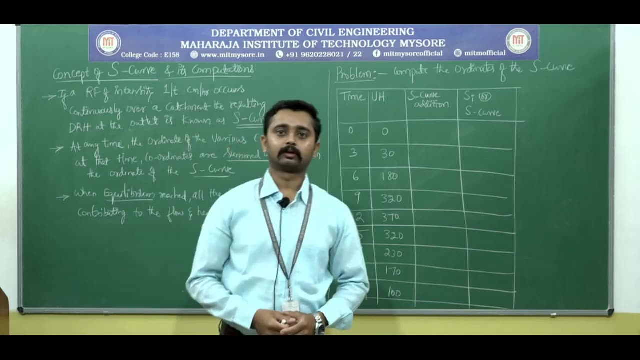 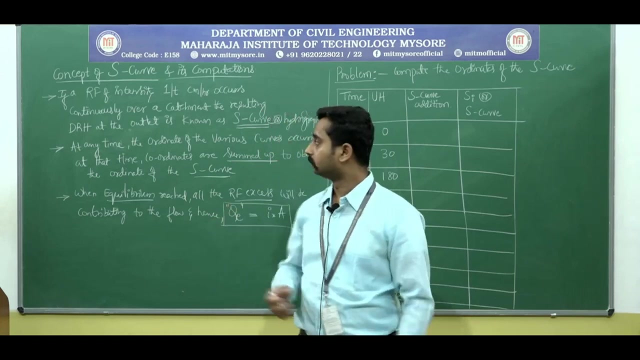 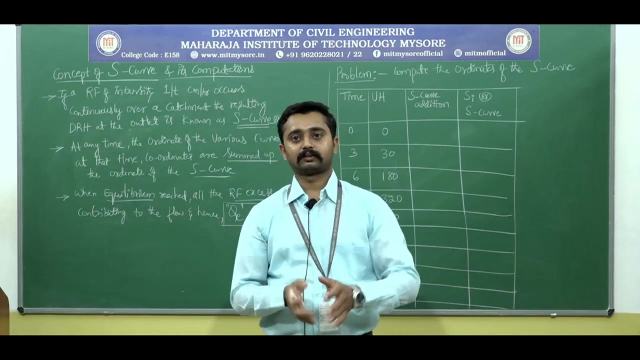 Okay, Thank you. Good morning. welcome to the new session. Today we are going to discuss about another small topic in hydrology, and that is in this module, that is, S curve, concept of S curve and its computation. Till last class we studied hydrograph, unit hydrograph and definitions. 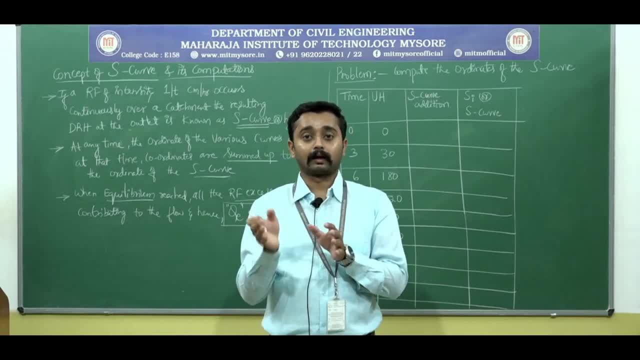 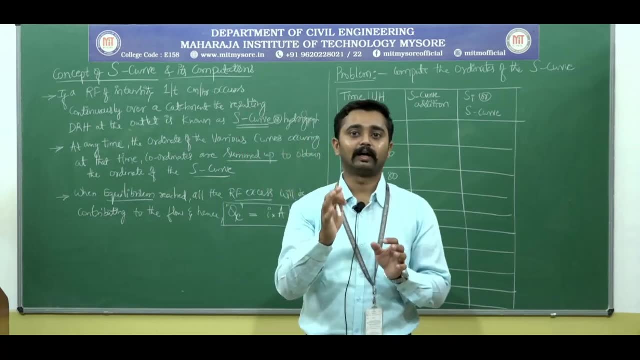 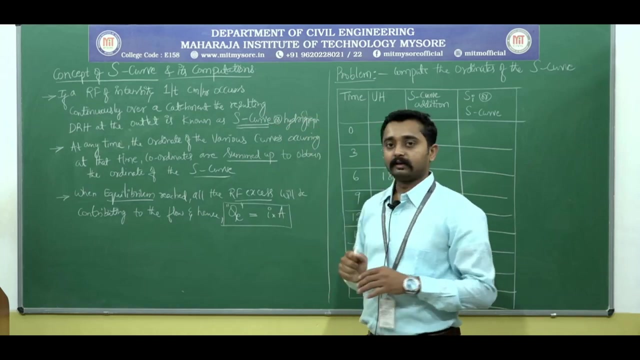 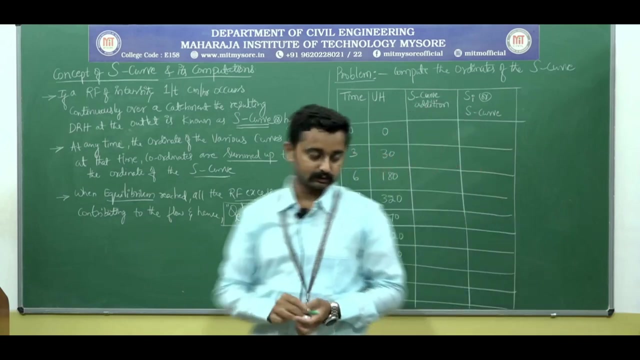 of direct runoff, hydrograph, surface runoff rainfall, excess and effective rainfall. So you should know very clearly, in order to understand the coming concepts Here, concept of S curve and its computation- Before entering into the theory part, just I will write one diagram carefully, see carefully. 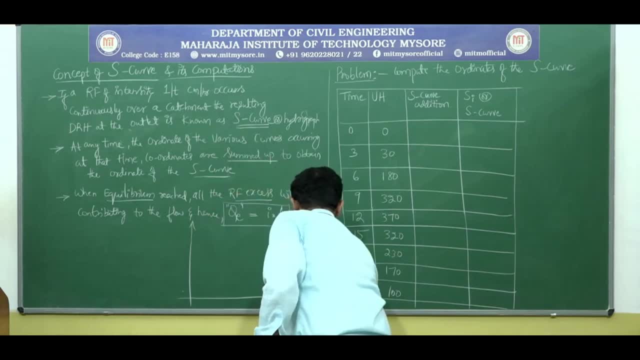 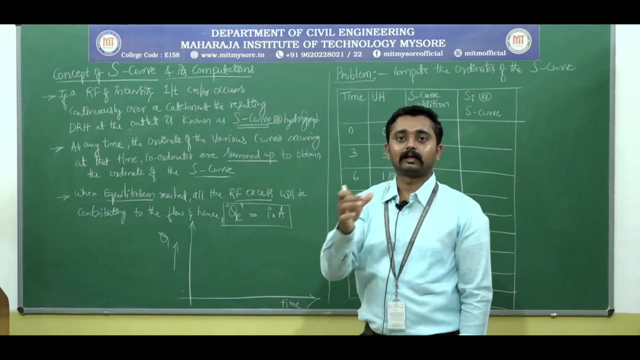 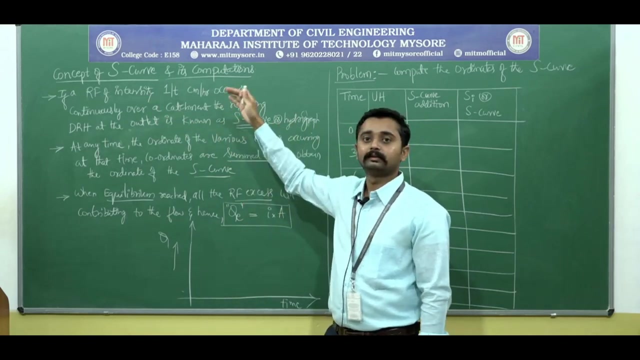 In X axis, there is a time. in Y axis, Q, nothing but discharge. Just listen, what exactly S curve if a rainfall of intensity, let us say 1 by T centimeter per hour, 1 by T centimeter per hour occurs? 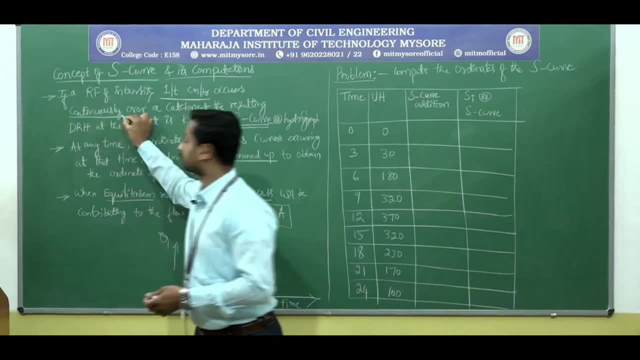 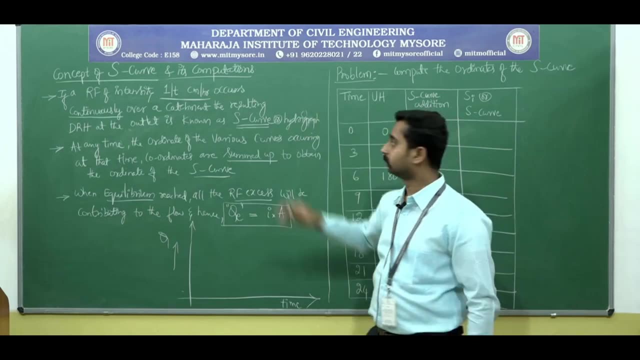 1 by T centimeter per hour occurs. 1 by T centimeter per hour occurs Continuously. this word is important. This is infinite number of time. So 1 by T centimeter per hour of rainfall intensity occurs continuously over a catchment. Let us say 1 by T centimeter. 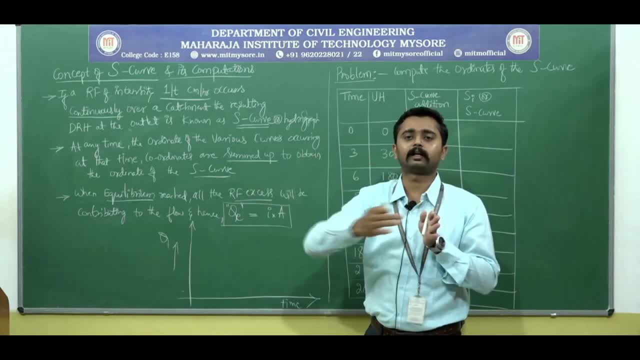 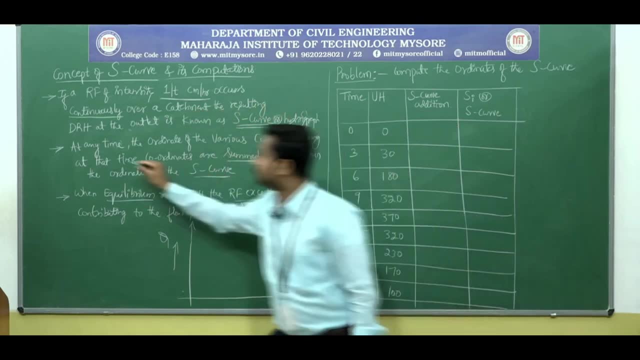 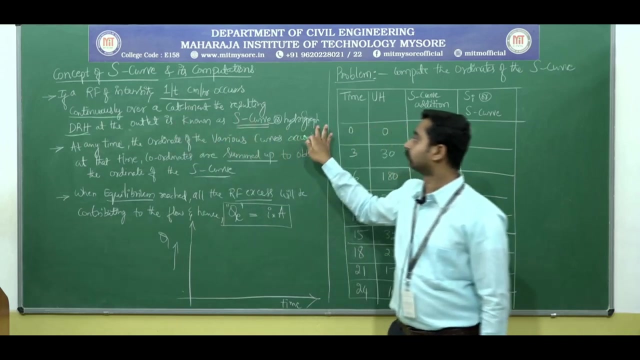 per hour of rainfall intensity is continuously, infinitely, continuously occurring over a catchment From that rainfall, the resulting direct runoff hydrograph, the resulting direct runoff hydrograph at the outlet is known as S curve or S hydrograph. I repeat once again: 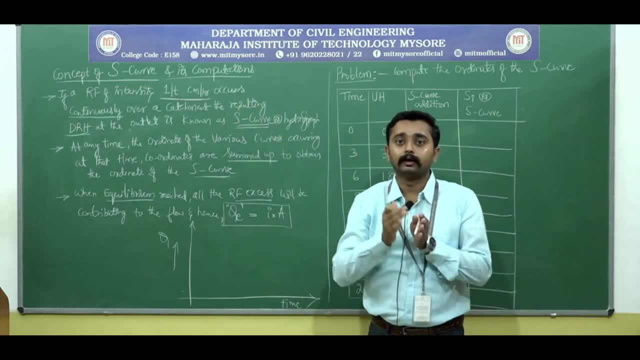 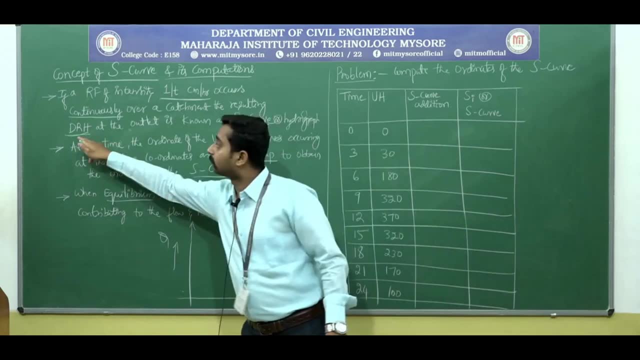 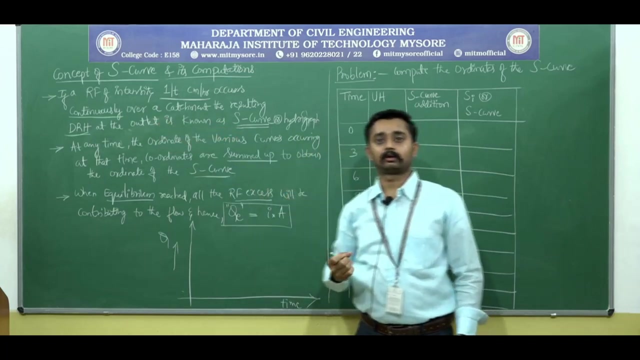 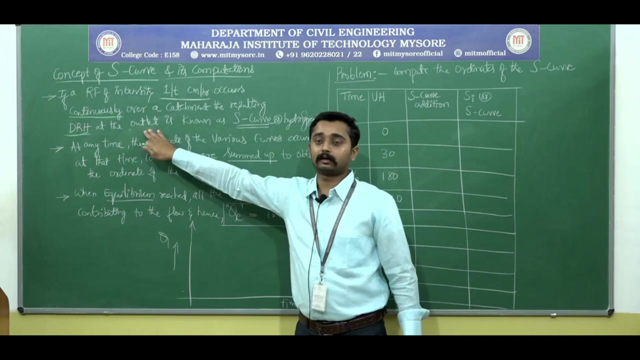 1 by T centimeter per hour of rainfall intensity continuously occurring over a catchment. From that, whatever, the direct runoff hydrograph is coming at the catchment outlet. at the catchment outlet, because of the rain fall intensity, we call that direct runoff hydrograph. 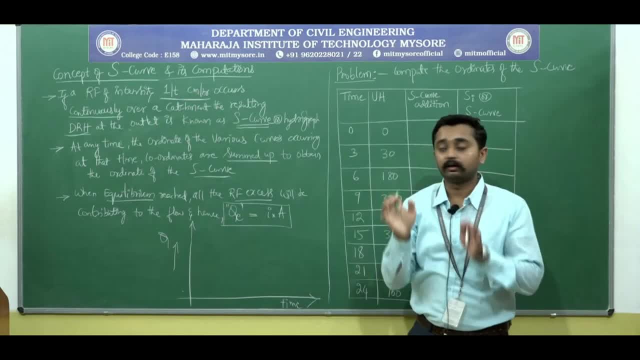 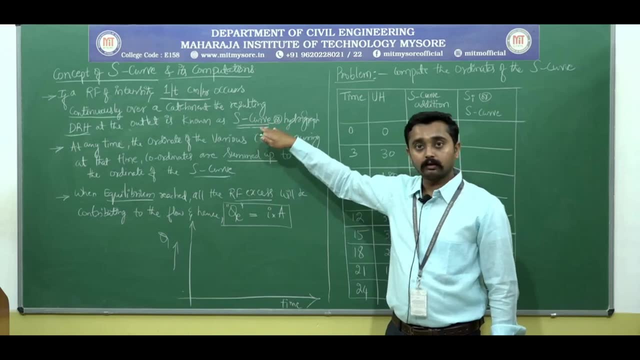 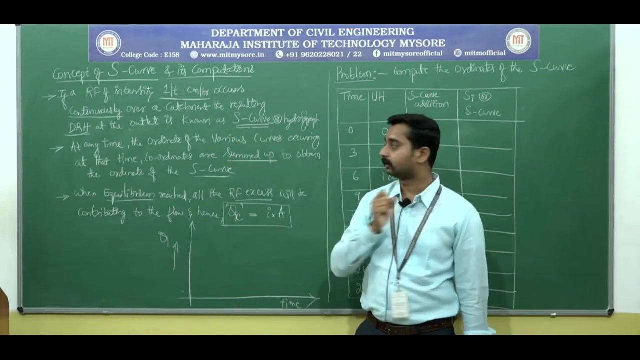 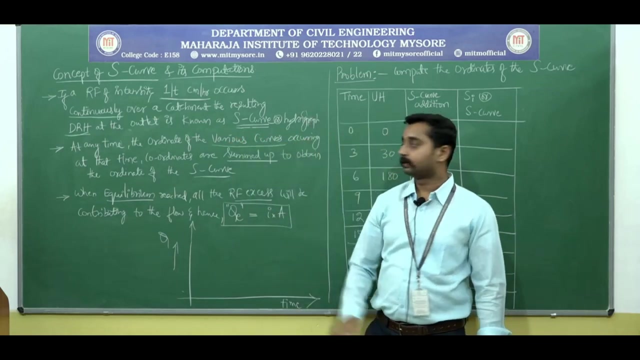 We are saying at the catchment outlet, because of the line for intensity, we call that direct runoff hydrograph. the obdinate of driven hydrograph is called as S curve. okay, At next point is, at any time, the ordinate of the various curves. at any time, the ordinate. 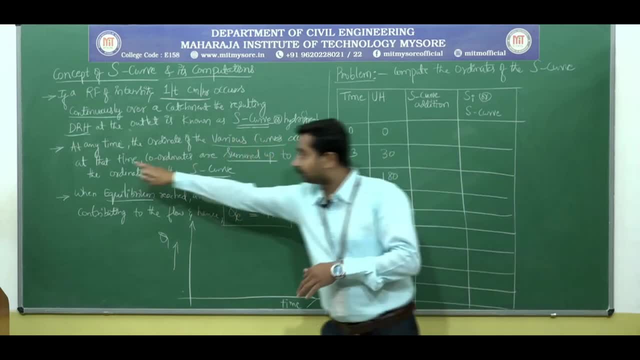 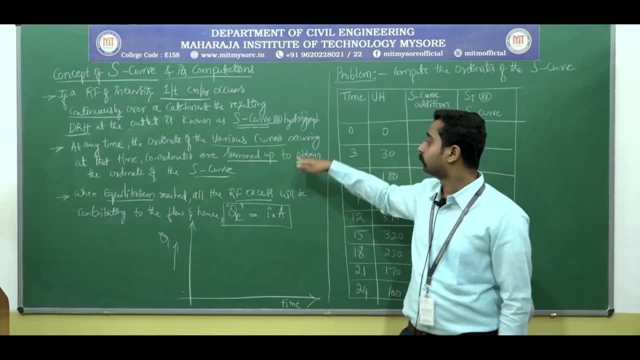 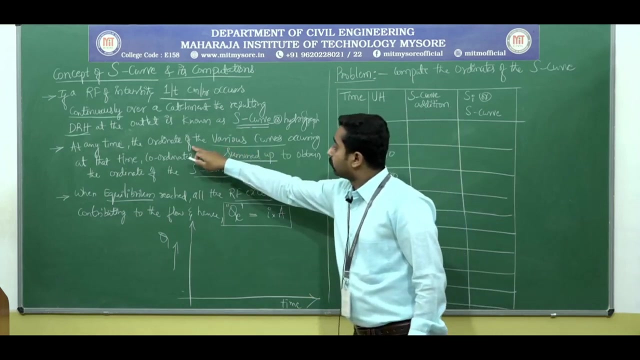 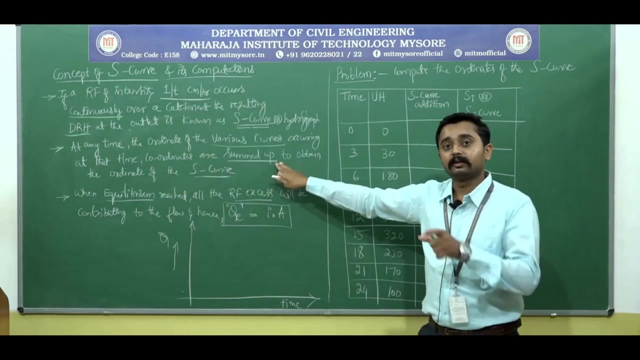 of the various curves occurring at that time. okay, coordinates are summed up. coordinates are summed up to obtain the ordinate of the S curve. okay, Now listen carefully, listen. this diagram: ordinate of the various curves occurring at that time. okay, we are summing. 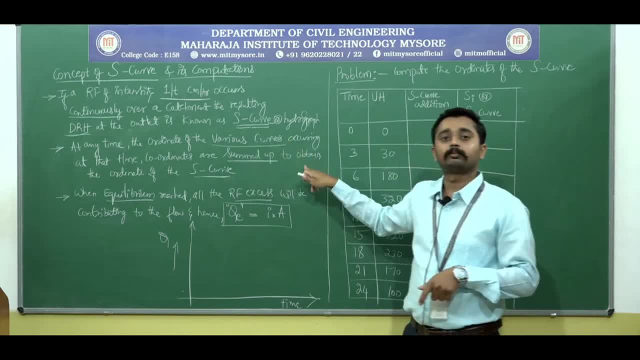 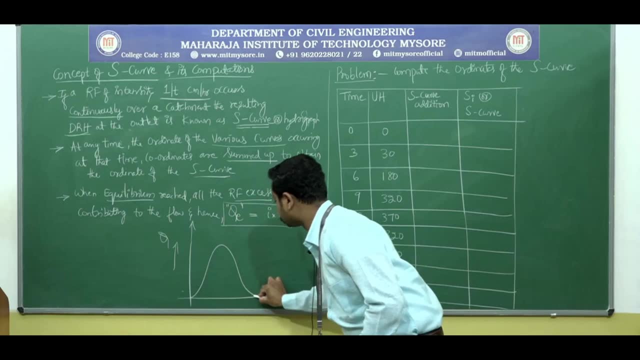 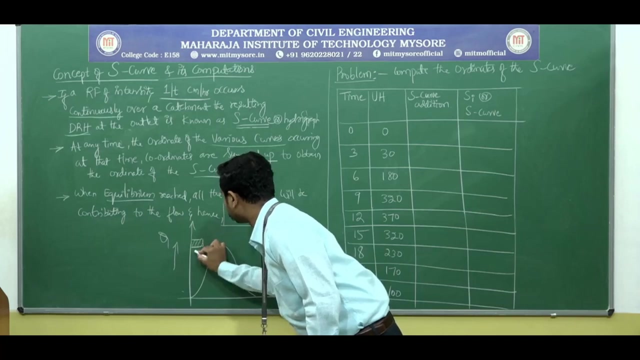 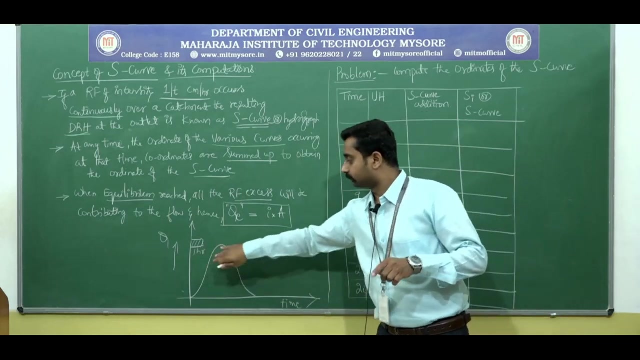 up. we are adding up these various curves to obtain the S curve ordinate. Let us say, for example: okay, this is a unit hydrograph. okay for 1 hour duration. okay for 1 hour duration, Rainfall intensity. I mean, this is 1 hour rainfall, this is the unit hydrograph. 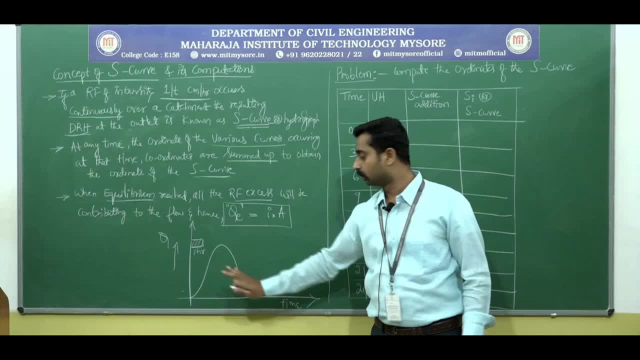 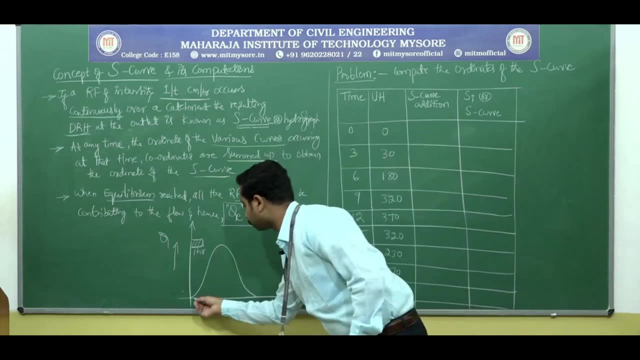 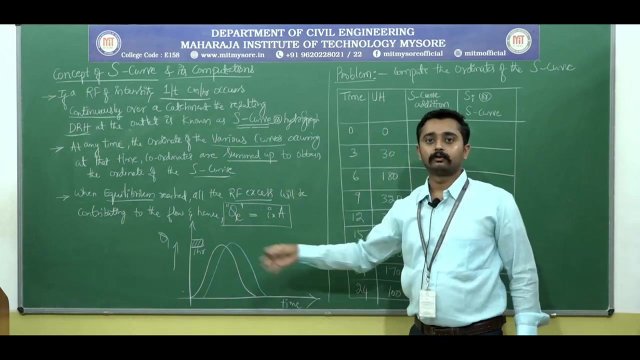 Unit hydrograph is nothing but 1 centimeter depth. That you must know. okay, After 1 hour there is another rainfall means another unit hydrograph After 1 hour. okay, this is another unit hydrograph. Next, after 1 hour, again, there is a rainfall. 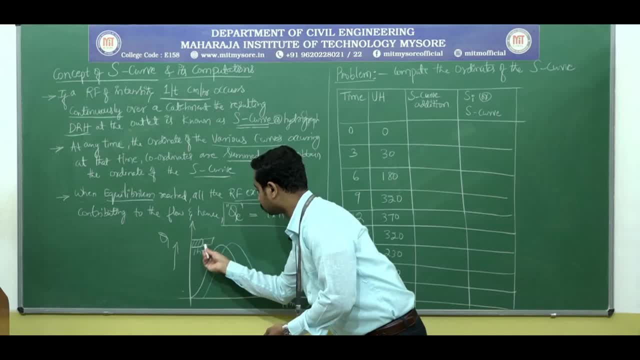 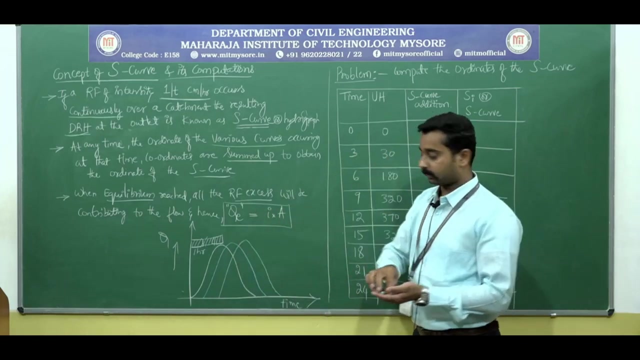 After 1 hour: okay, after 1 hour, there is again rainfall. Next after 1 hour: okay, this is another unit hydrograph. Again after 1 hour, again after 1 hour, again after 1 hour, there is rainfall. 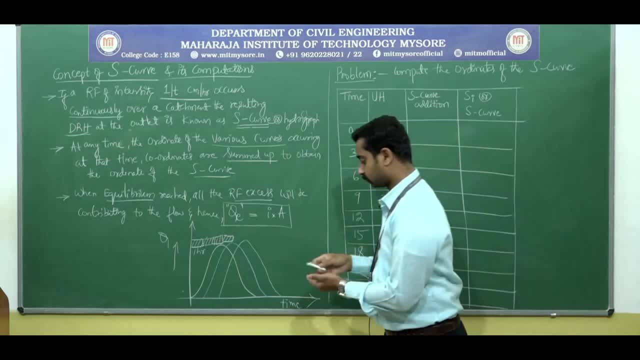 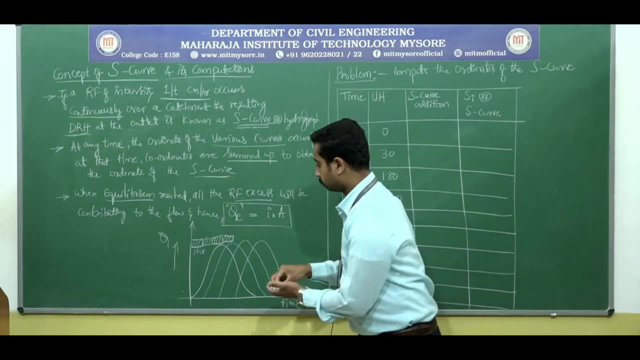 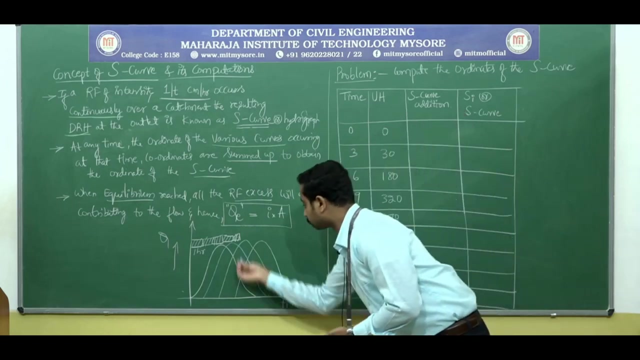 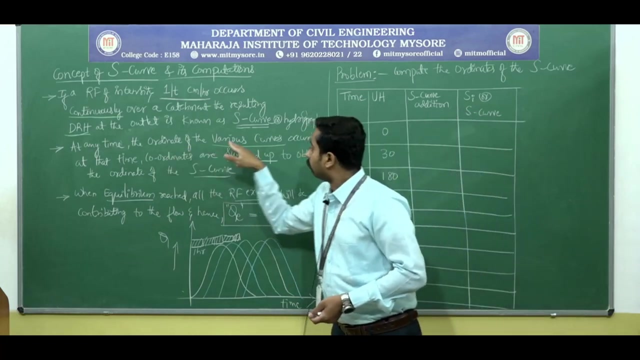 So the next curve, next unit hydrograph is like this: Again after 1 hour, again after 1 hour there is a rainfall. okay, again after 1 hour there is a rainfall. So time, this is another unit adder graph. Now various curves occurring means the: 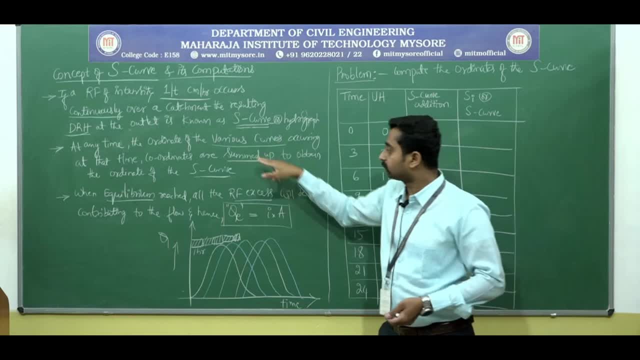 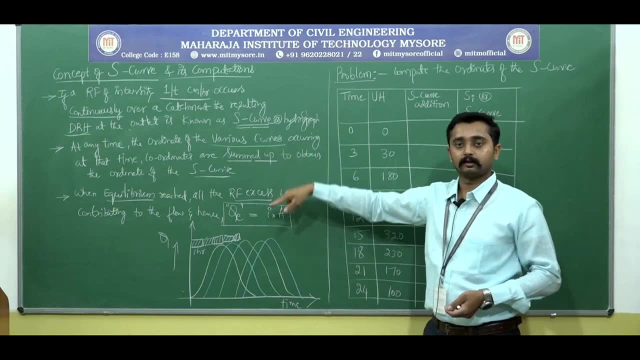 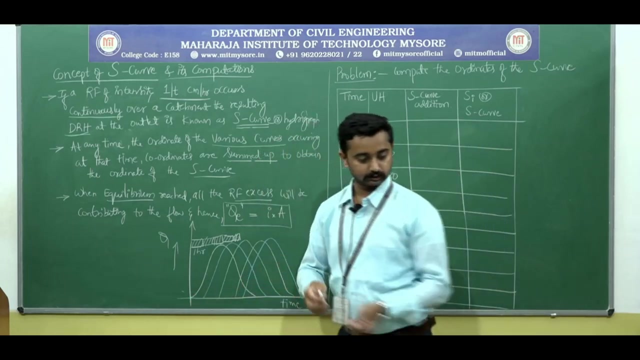 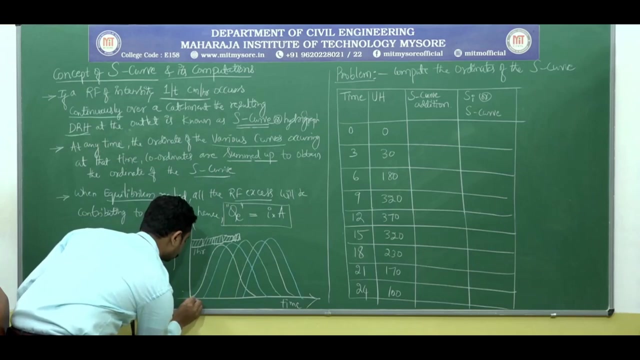 ordinates of the various curve. if we summed up, if we summed up all these ordinates, if we summed up adding up all these ordinates, we will get. we will get. okay, this is the ordinate of the s curve. the yellow line: ok, this is the yellow line. listen carefully. after adding all the 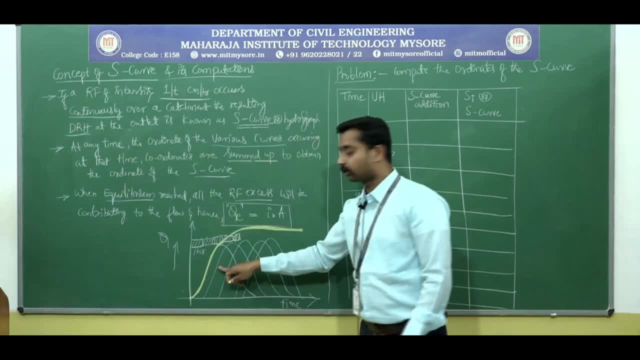 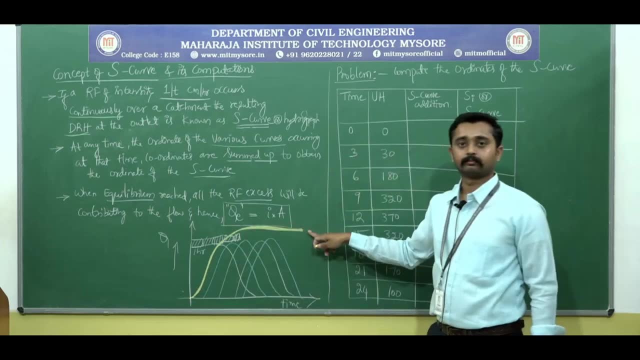 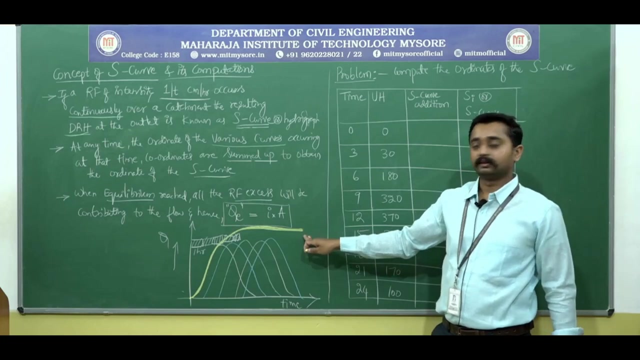 ordinate of individual unit adder graph. After routing all the ordinates of these curves, you will get a curve like this. You will get curve like this. This is what in the form of, in the shape of S curve. That is the reason why we call this as S curve hydrograph. 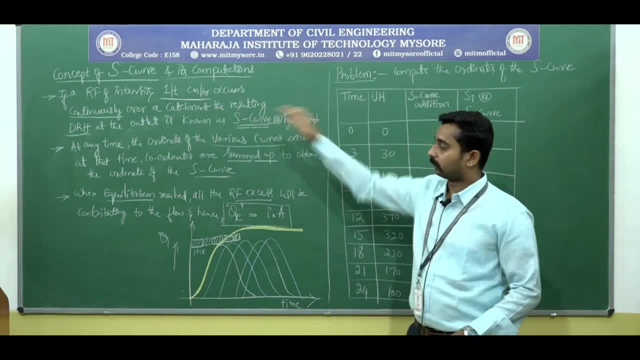 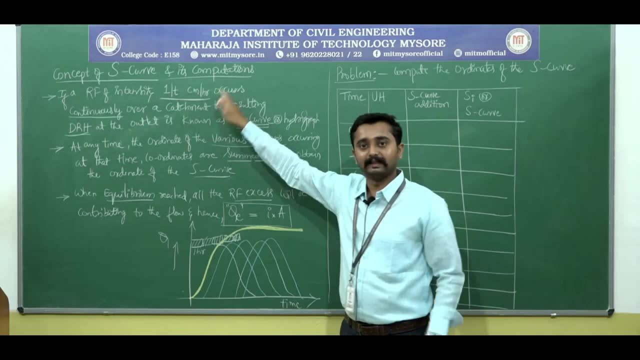 Okay, Just what is S curve? 1 by T- centimeter of rainfall. 1 by T, Let's say, for example, 1 by T centimeter of rainfall intensity occurring over a catchment continuously. The word is important: Continuously. 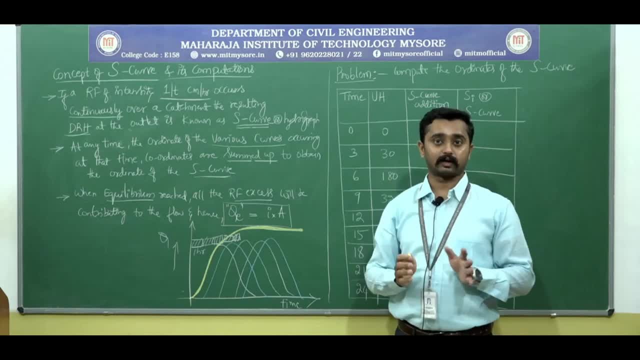 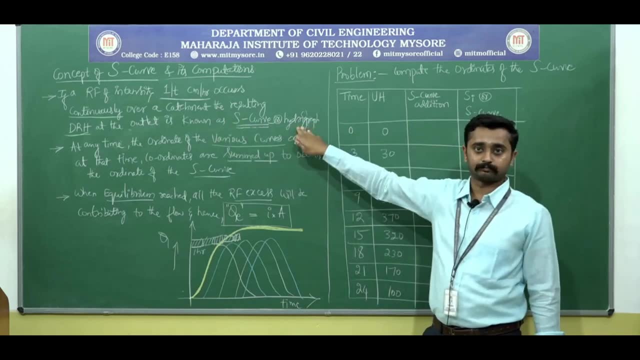 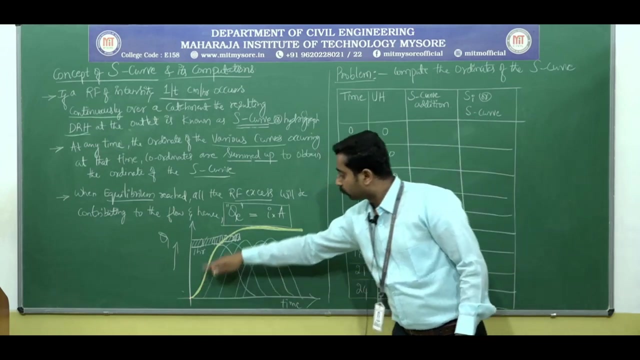 Okay, From that the resulting direct runoff hydrograph, the resulting discharge is called S curve or S hydrograph. Okay, Just by adding the individual curves unit hydrograph, we will obtain the ordinate Of the S curve. Okay, 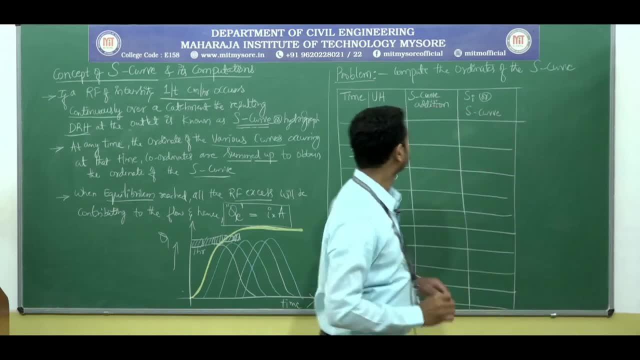 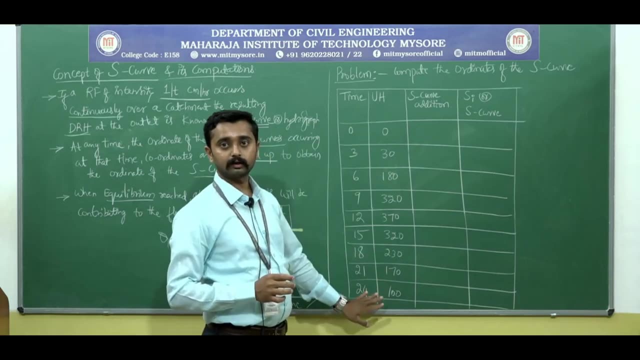 Now just take a simple problem to understand this concept: Time 0,, 3,, 6,, 9.. Okay, This is the given data. Unit hydrograph is given. Okay, Unit hydrograph is given. Now just add up. 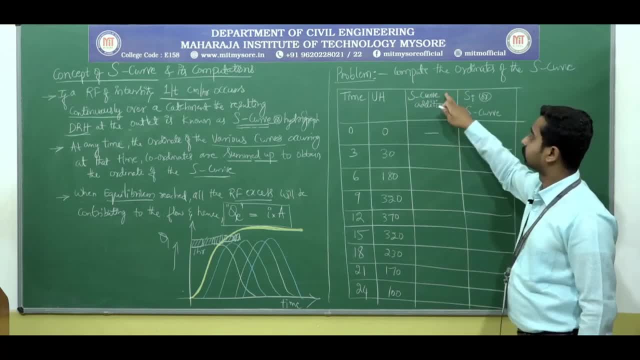 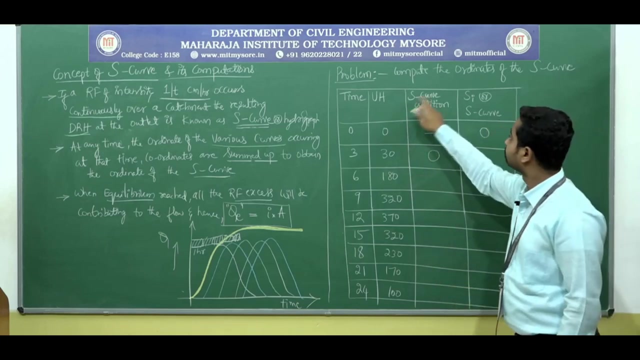 First I will write- this is third column- is S curve addition. Fourth one is S curve, represented by S First value. write as it is. Okay, Just replace this. 0 here Means S curve addition. So this is the lag time.